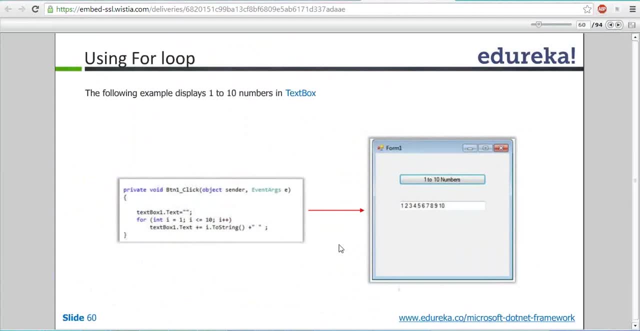 button. I want to display the one, two, ten numbers in the text box. Same thing, I'll do. Text box one dot text equal to initially nothing. I'm grouping Here. I'm writing: I equal to one, I less than or equal to ten, I plus, plus. Text box one dot text plus is equal to That. 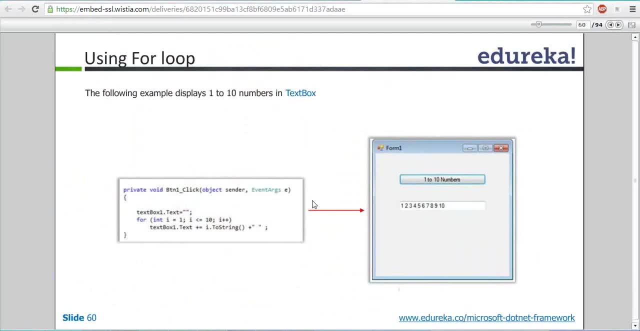 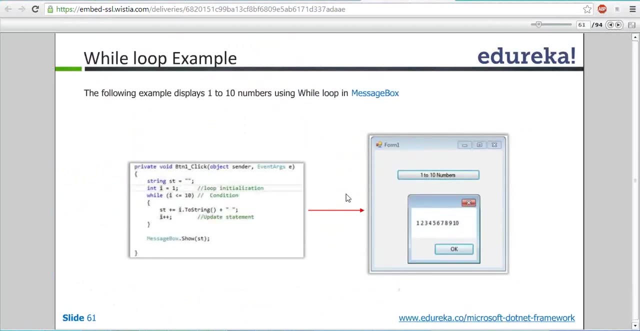 empty text is going to be adding with one, two, three, four, five, So the output will be like this: Okay, So loops can be implemented here also. Let's see this Here: same thing using the. I took one string variable. I is equal to zero. I equal to one, I less than or equal. 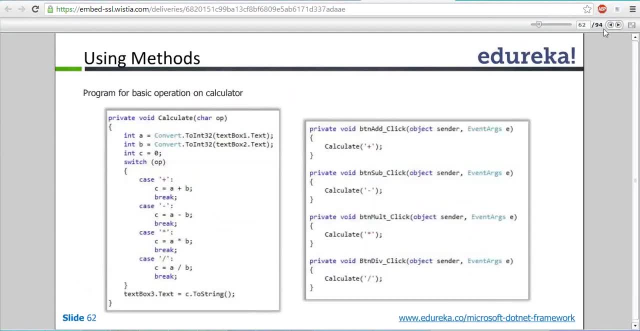 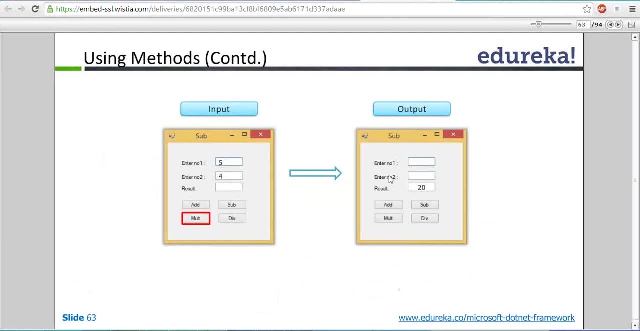 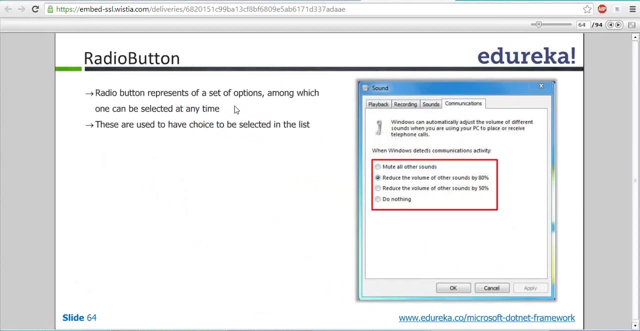 to I plus plus Right Here, same example, which is multiple screen. The screen contains multiple options. When you click on any option, the respective action will be performed. Four buttons are calling the four definitions. Now, okay, radio button. So what is a radio? 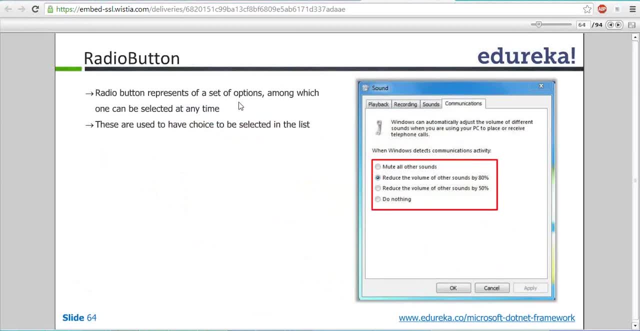 button. A radio button is used to place multiple options and allows to select multiple options. Any button Radio button is used to place multiple options and allows to select one. Okay, See something called as a question paper and in every question paper object. 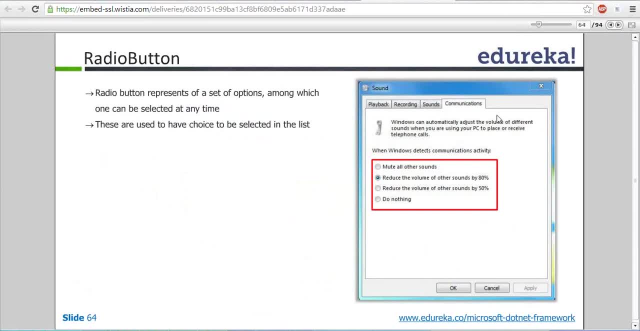 question. You'll be having one question and four options. One question and four options. You are allowed to select only one, So the best choice is radio button. Okay, So radio button is used to place set of options and allows to select one. Okay, Check box See. 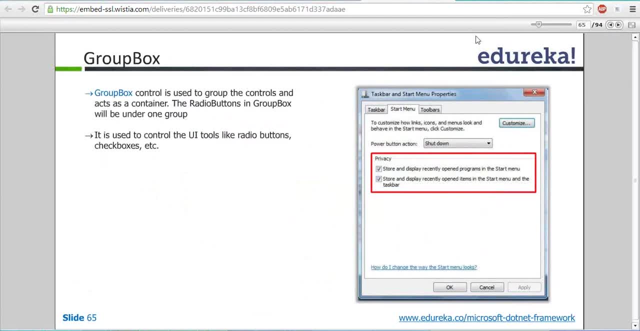 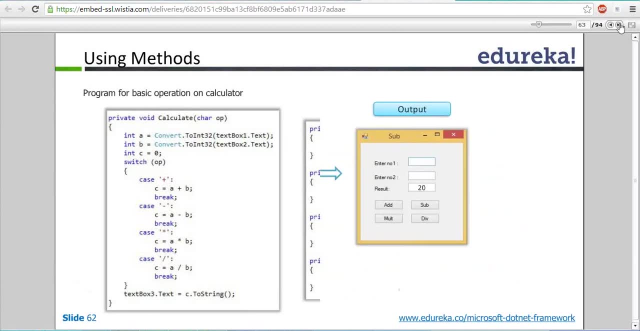 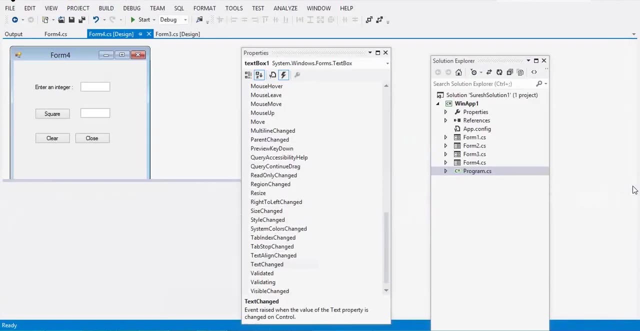 check box group box. Group box is used to group. the controls Group box is used to group. Let's come to the next one. as I said earlier, we can have the loops, we can have anything, Let's see. satisfaction will have one loop while the other one is following my own. very. 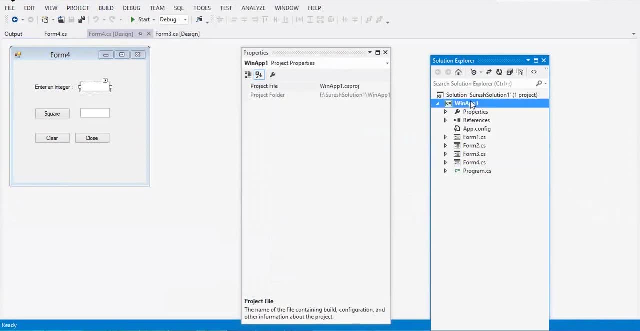 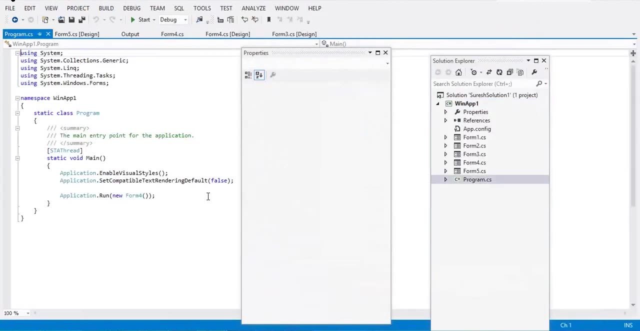 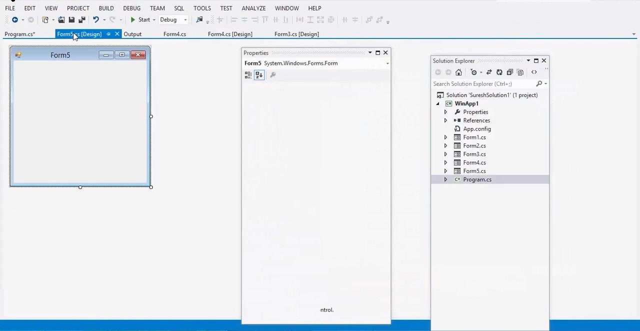 small program. Let's see this. Add a form. Add a form. Please select the form. go to the program. just change the number to 5.. Here you have the 5th form. let's see the 5th form. here I'm having a label. I would. 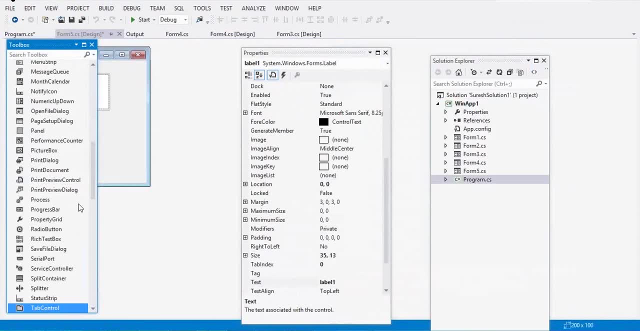 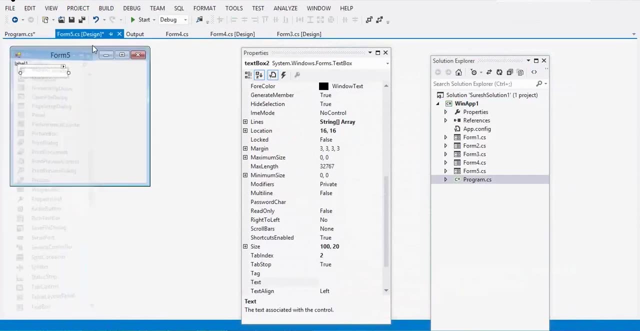 like to have the table. sorry, I was mistaken the text box. What is my question here is? this is for displaying the output. If you want to make a multiple, you need to select a multi-line and you need to select. 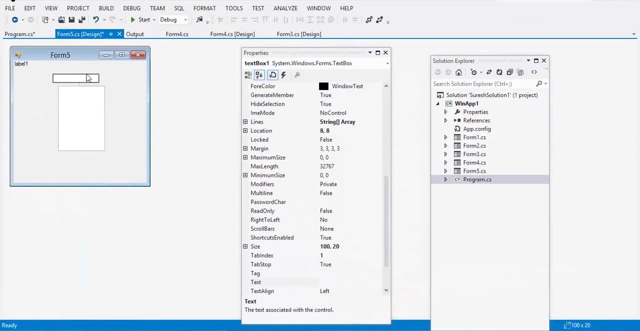 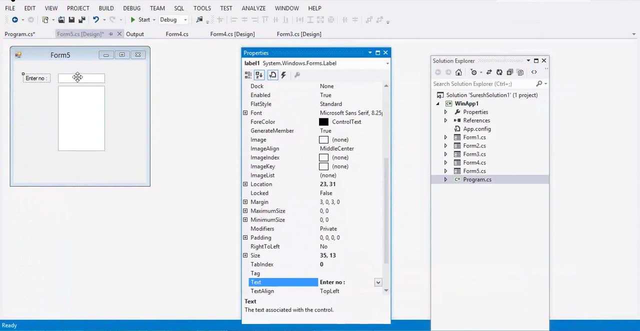 this. This is multi-line. What is my question here? I would like to have an enter number. See, I'm asking enter number right now when I enter the number here. now I would like to have a button. So what is the button? 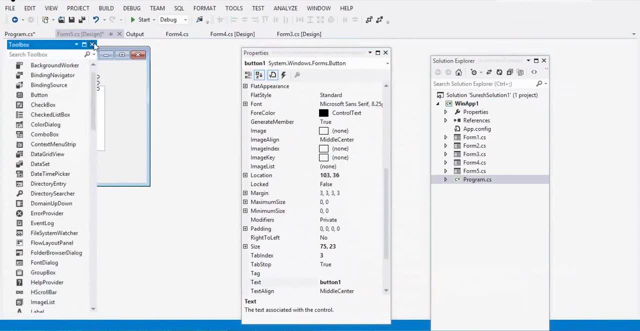 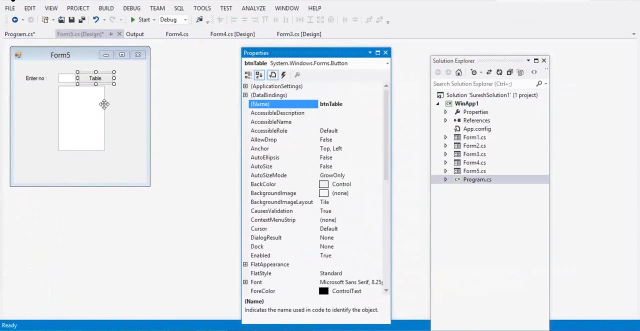 I want to generate a multiplication table, so I would like to have a table. So when I click on this button, I would like to generate a table. So this table should be generated when I click on this button. Let's see this. 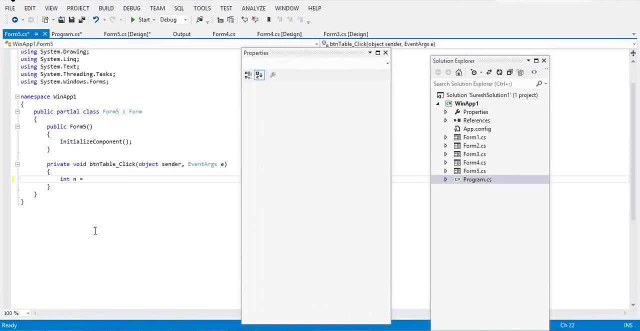 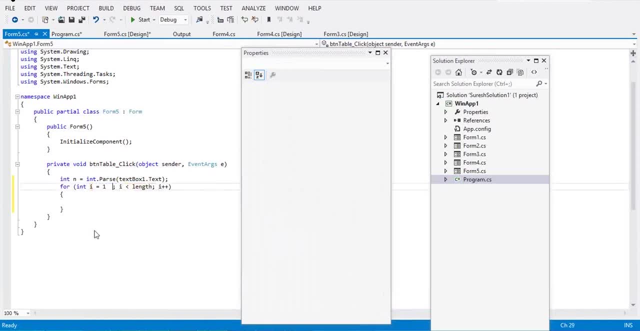 I want to generate this. that's perfect. So for I is equal to 1, I know this. i less than or equal to 10.. Okay, i less than or equal to 10, no, here I'm making. Okay. 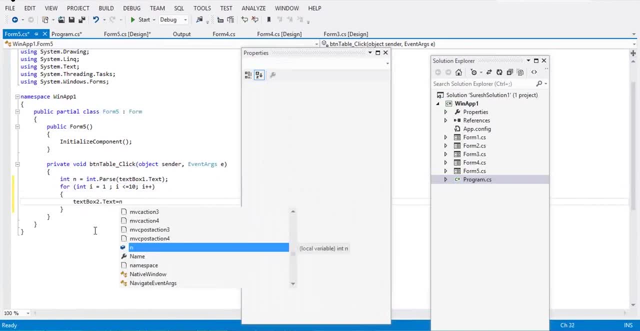 Textbox: two dot text is equal to N. Okay, And what I want to have? um say it's 6. 6. Now I want to have the n dot toString now. next, I would like to have n followed by some. 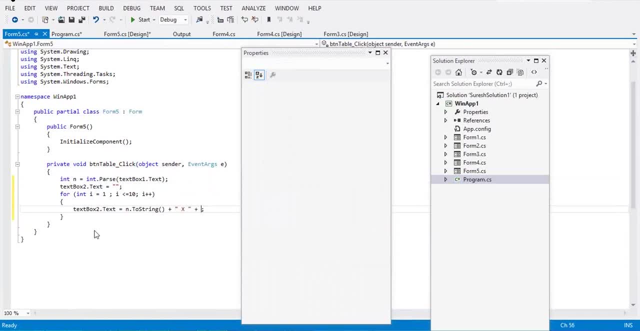 star symbol into symbol, followed by i dot toString. now n into i dot toString is equal to symbol, so I would like to have this equal to symbol n into i dot toString. let me check this now: 1x squared is going to be x squared. yes, it is. I give 6, click on the button. 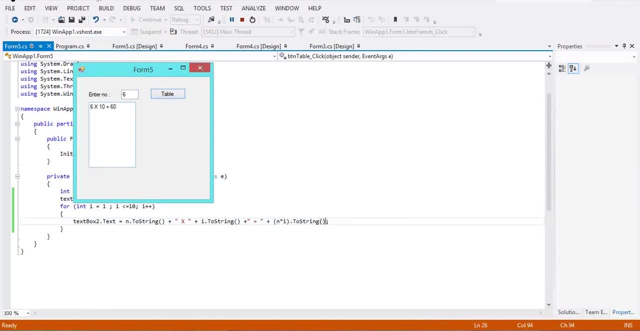 6 equal to 10, now existing value to be added right plus is equal to: let's execute this: 7, 7, it's coming. I want to get the next line. how do I get the next line? let me check. 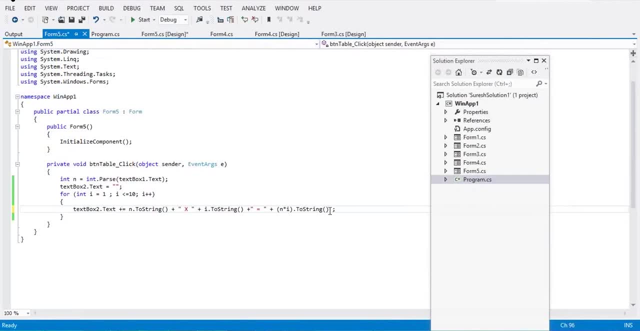 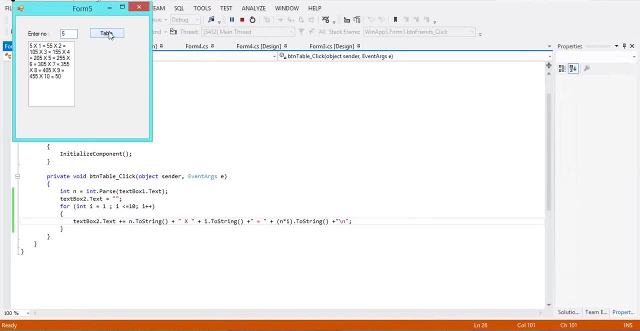 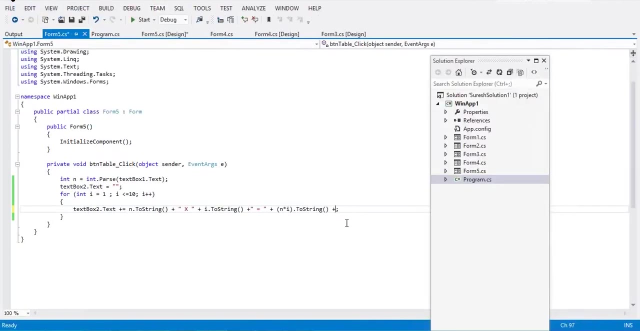 it. first Let's pop 902 and the next line plus symbol, slash n. let's execute this. this file now. plus symbol is not accepted. to give this one how to go to the next line: 991, string dot n. text box dot n. 991, next document. 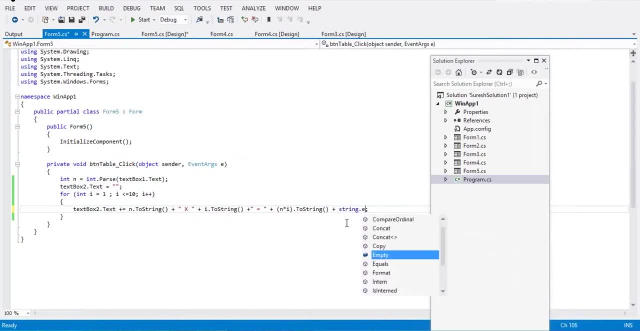 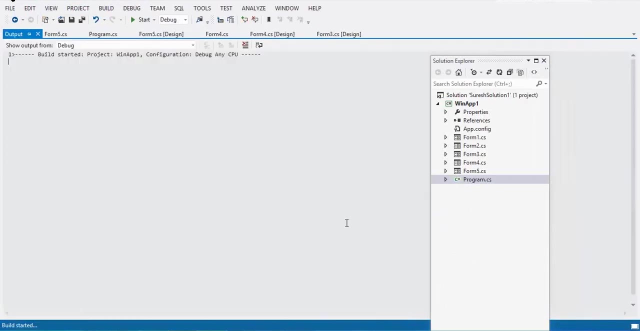 Can I check it? I cannot generate a blank. I have to check how to generate a blank, blank, blank, blank. Anyhow, no. issue three: you can do it. six, six, table now. what you do is just to reduce. 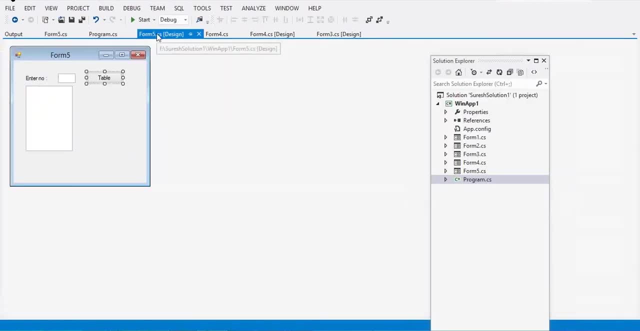 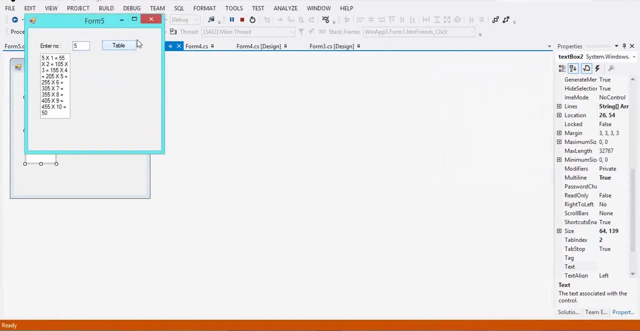 the size to something. now change the size, let's execute it so it's exactly the same as six. six table, five table. just reduce some things. I can do some here, but we can do some space also. six into one equals six. it's just a small change. I forgot here how. 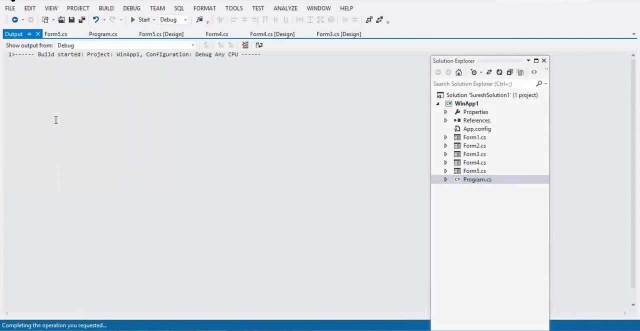 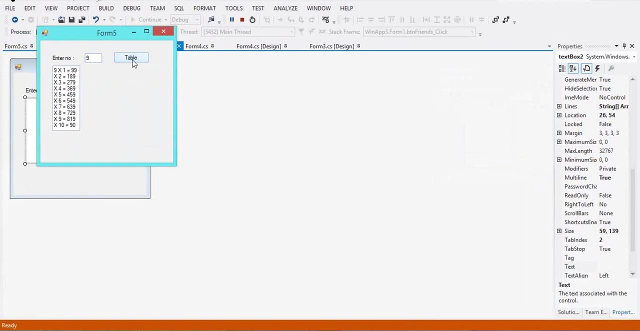 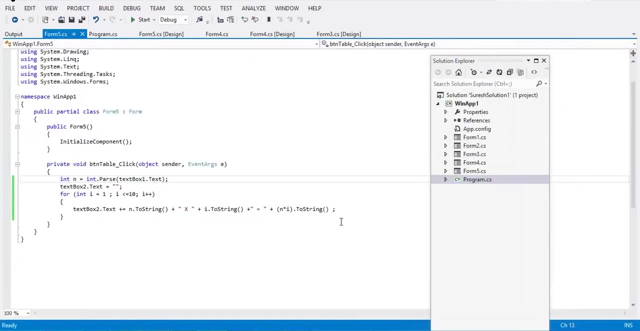 to do? we can actually do it. some string dot in D line or something, is there six, nine, nine into two equals ten, nine into two equals ten. One second. I'll tell you one suggestion: let's get the tab space. so six, okay, you. 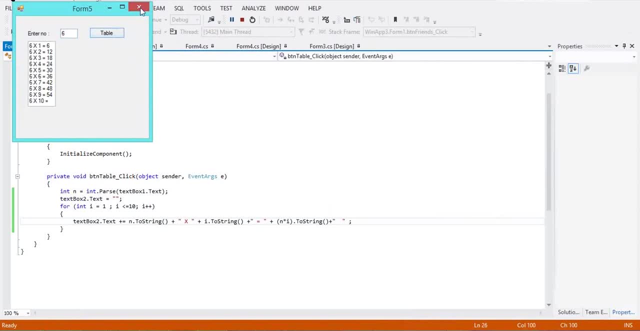 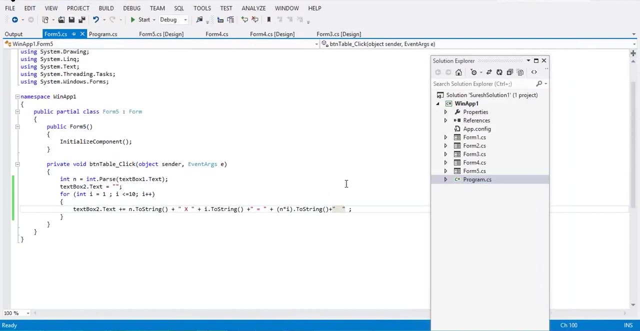 can get that. okay, you can have that. okay. a multiplication table can be easily. so what I mean to say is your arithmetic operations, loops etc. can be okay. you can use ASCII value. ASCII value is 13 is ASCII value. can you use ASCII? 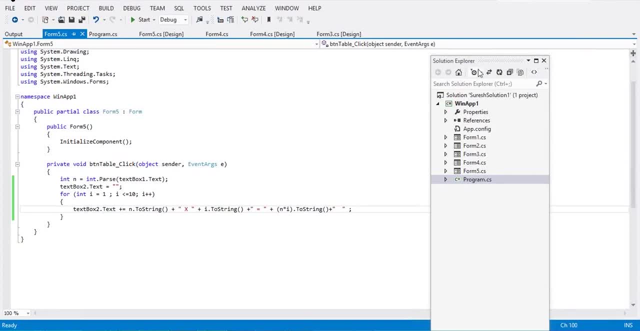 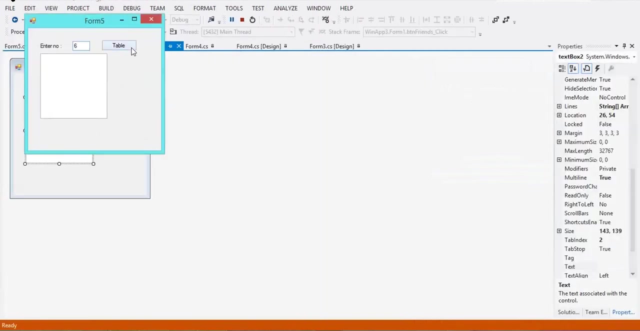 value, I think, Environ. yes, Environ, it is accessible. I forgot. okay, thank you, Environ. Let's see this all right. absolutely so. let me check whether it's working or not. Google is there right? very good, right. absolutely okay, it's working, yes, okay. 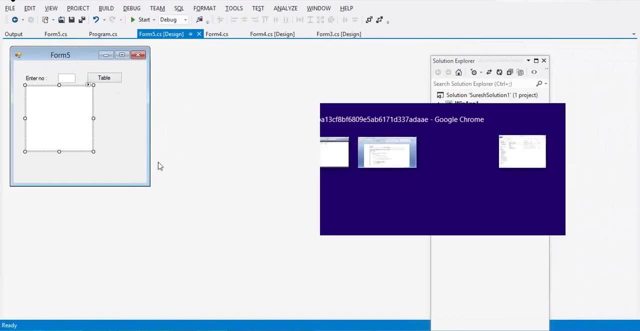 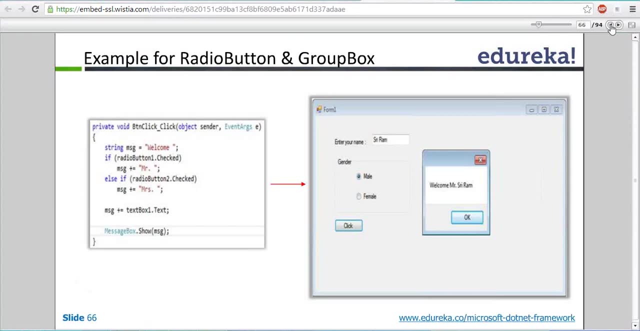 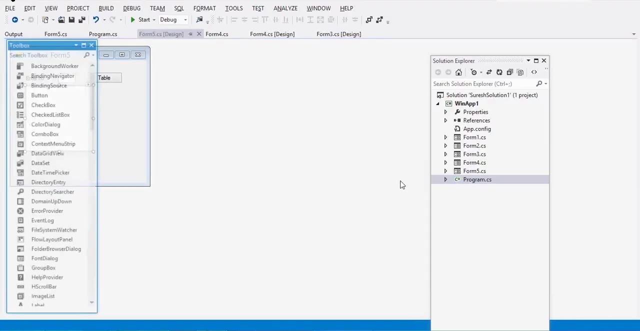 and in the end, this will be accessible using the Environ. Right now, what is this radio button? so radio button is a place where you can have multiple options. let's say this: this is very, very important here. you can see this right. 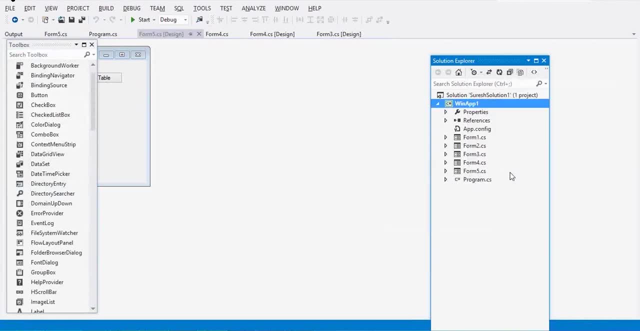 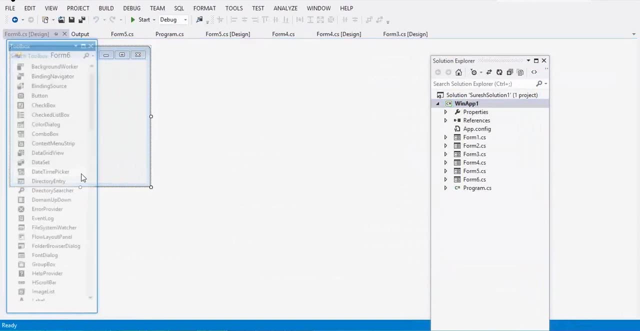 all right, okay, new icon. okay, so you can have this radio button. what is a radio button? radio button is an option button. see, I have a radio button. I want to place one more button, two, okay, so radio button is a place where we will be having the multiple options. okay. 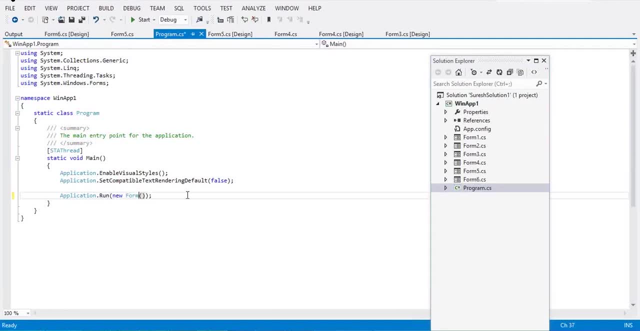 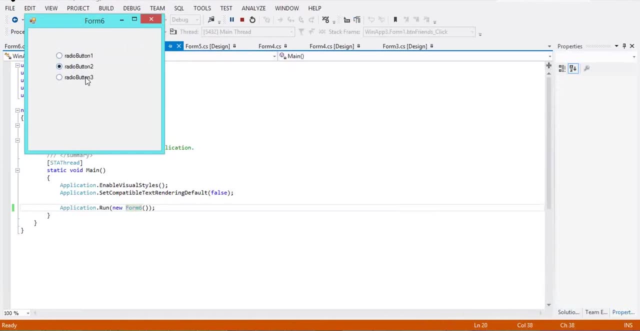 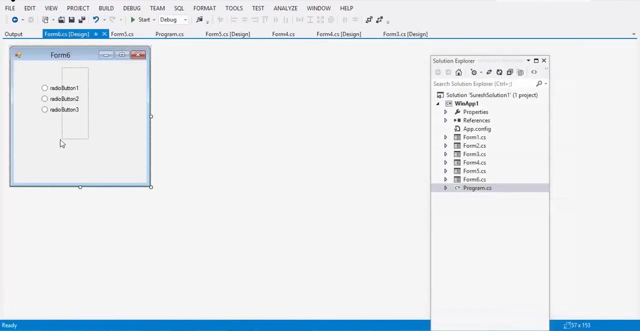 radio button is used to place multiple options, but allows to select only one. do you remember it's going to be So? this is what exactly call as Now, do remember what happen if you have two sets. This is one set and I have two, one more set. So this is. 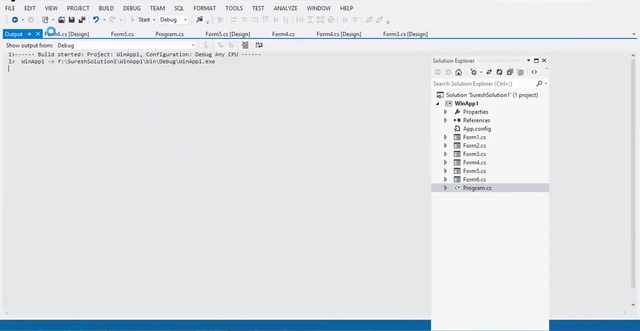 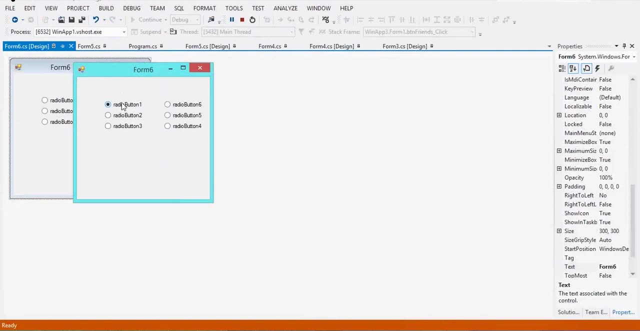 another set. I have two sets. let's execute it, But what happens? you know, all these are by default one category, So this is a problem. All the buttons will be under one category. So how to make them different categories? 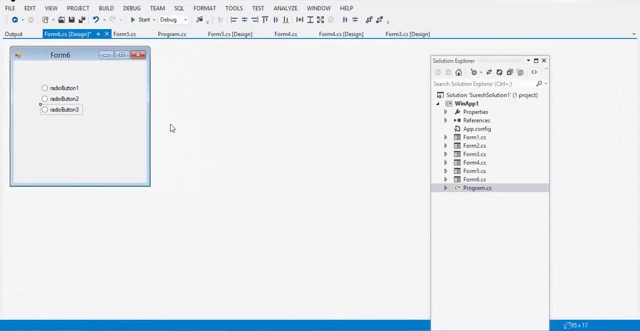 For this. in order to that one, we have a facility called as Groovebox. So what we need to do is put a Groovebox first of all. This is a Groovebox, And Groovebox is a place where you can have group of countries. Groovebox is a place where you can have group of countries. 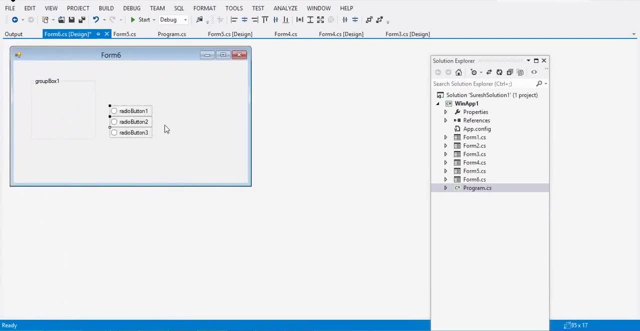 This is, first of all, place this until it's cut right. click on here, paste it here. Now what happens? you know this will be. Now you can understand these three really wouldn't have the group of these three. 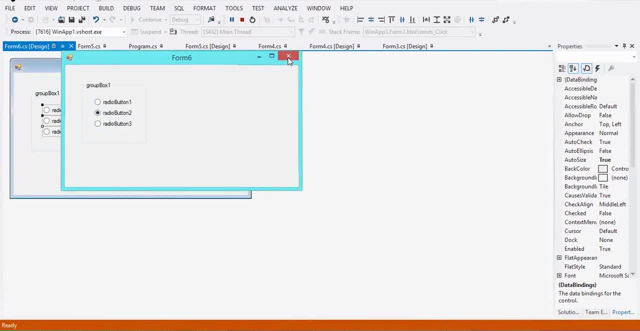 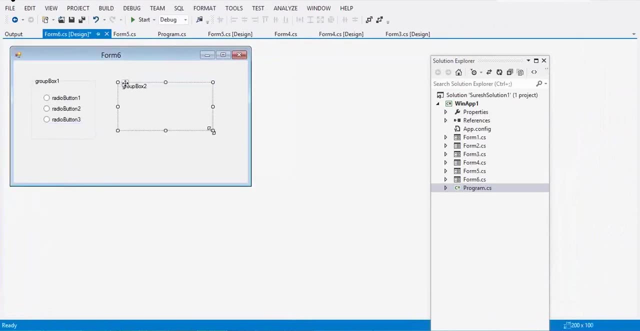 I will paste, I will paste. I will place one button Groovebox and in the Groovebox I will paste whatever example. I will copy this here: right click and paste. Now you can understand this. you know Now what I will use. I will have another Groovebox here. 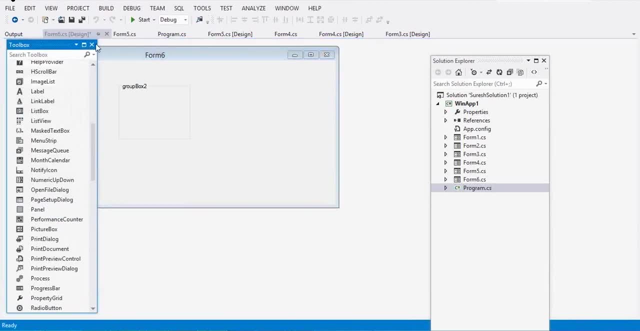 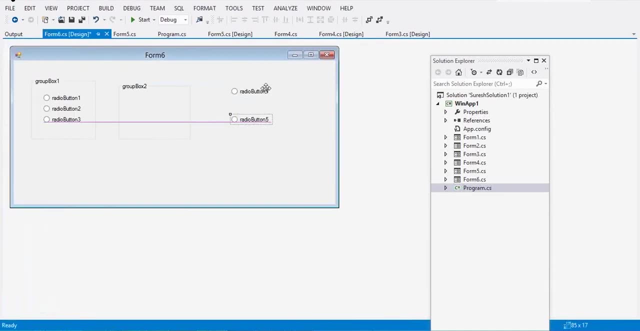 one example: I have a radio button, radio button four, radio button five. I have a radio button six. Let's copy this three. copy this three: control X, cut right click on this, paste Now what happens. you know, these three will be in the disk group and these three will be in. 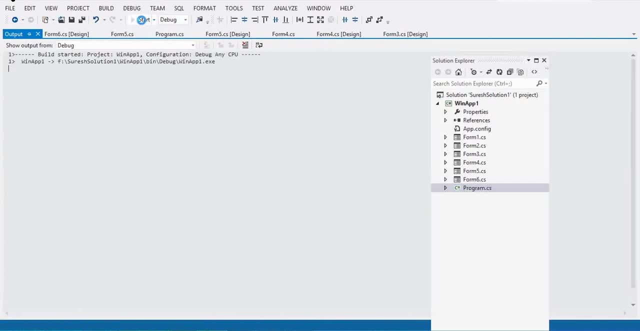 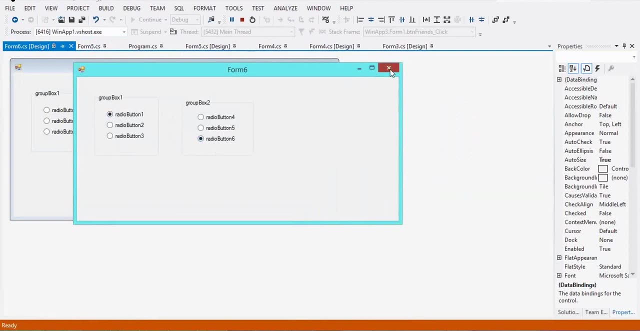 the disk group. Let's click on this so you can see this. See how to group the radio buttons. You have to use this. Have an idea? Great, And how to handle the radio Radio button. dot checker property. Radio button is used. 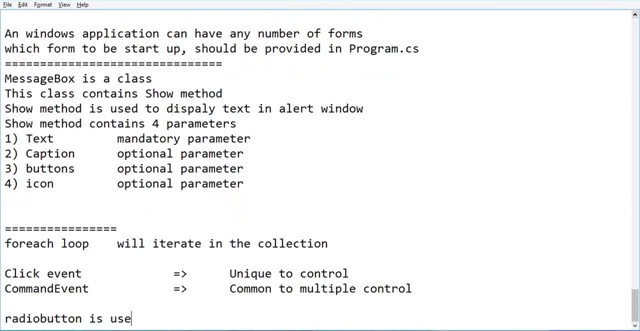 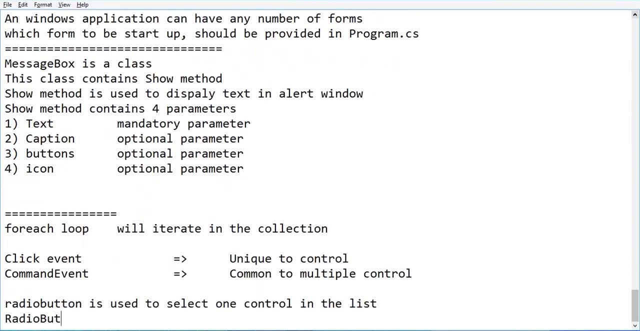 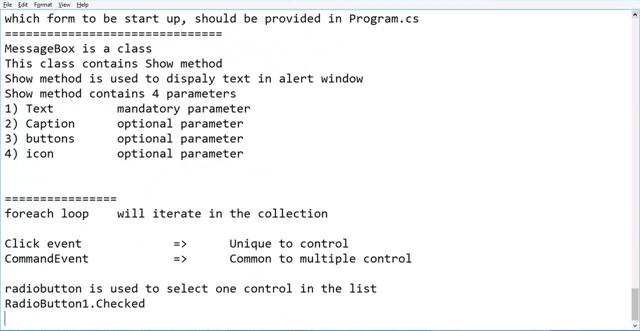 to have multiple controls. Radio button is used to select one control in the list. How to handle this Radio button? one dot checker. So checker is a property used to check which one is set and property Property control if the button in the radio button is set. 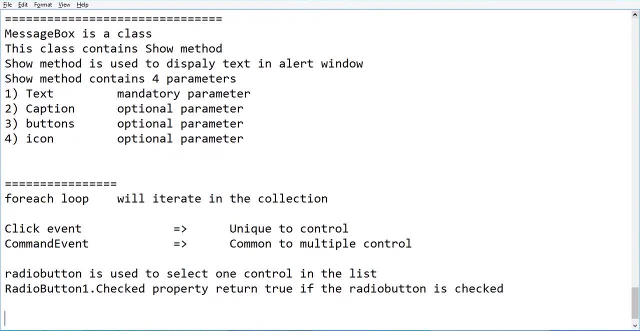 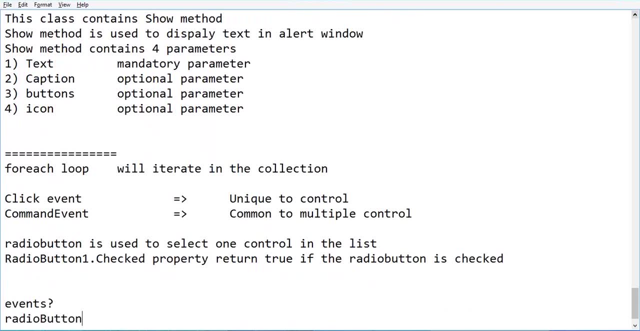 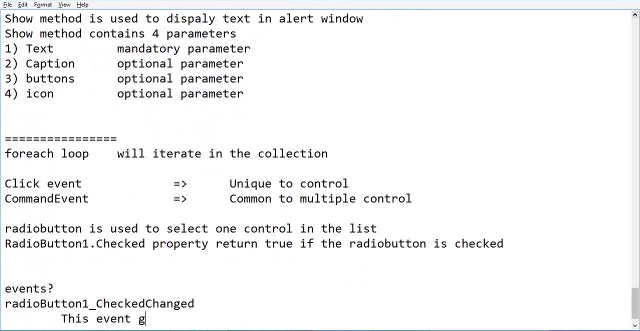 is set Right, The next one, If you want. even I want to do what is even The radio button, one underscore checker will change again, So you can understand. this gets released when the radio button is set, So you can do this. 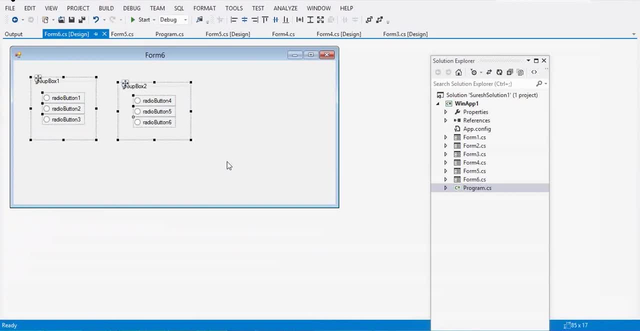 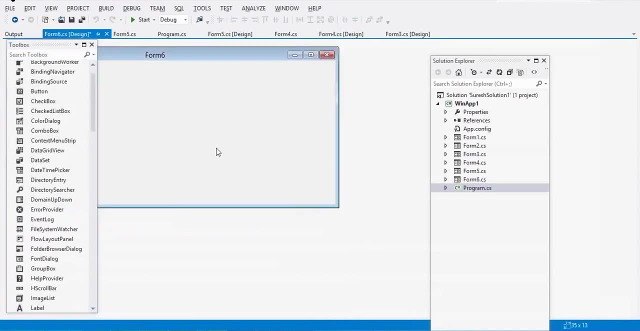 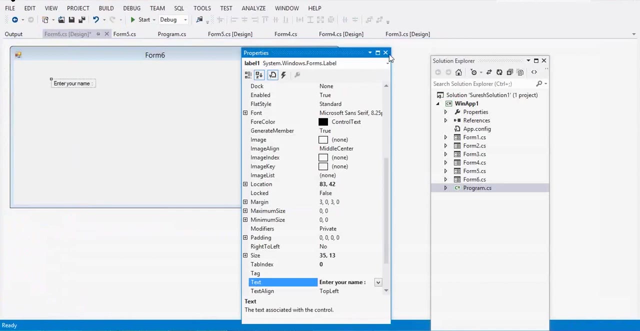 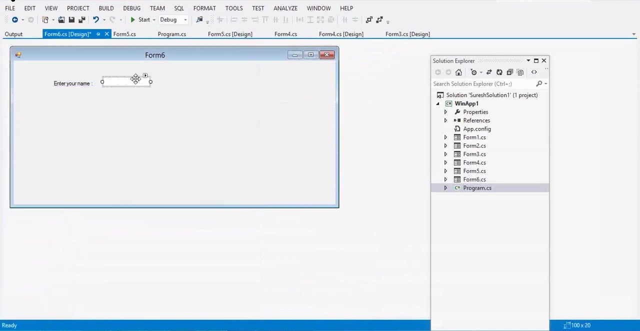 Ok, I'll remove all those things. I'll take a label and here I'm asking you to enter your name. Now here I have one text box. so in the text box I'm asking you to enter your name. Now what I'm doing is I have a group box. in the group box I'm giving some message called. 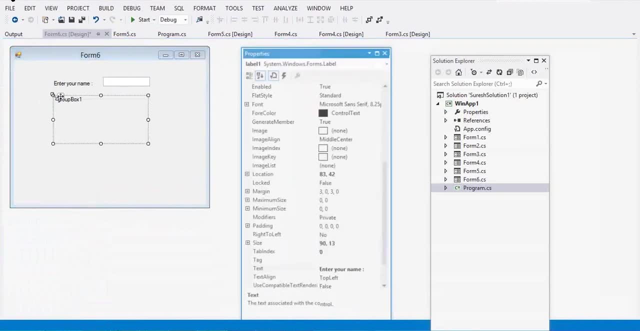 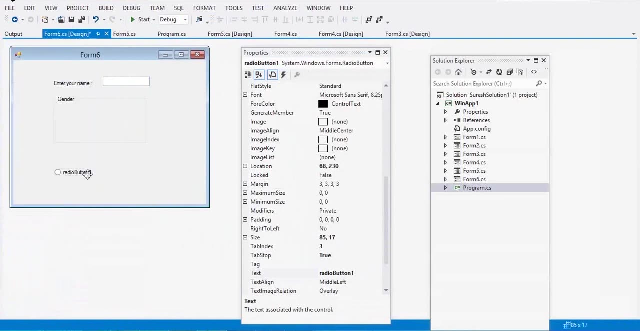 gender. select this as a text: gender and generally. when you're talking about gender, you have two radio buttons. one is the first radio button. select it. it's a male and the second one is female. Let's copy these two. okay, control X cut. now I define this text. it will be in two. 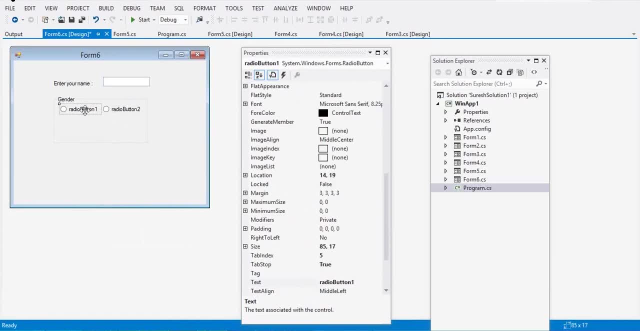 radio buttons. First one is gender text to male, gender text to female, and the names are very, very clear. the names are radio button 1 and radio button 2.. Now, here I'll put a button. so here, what is my question is, I'll be placing a button and 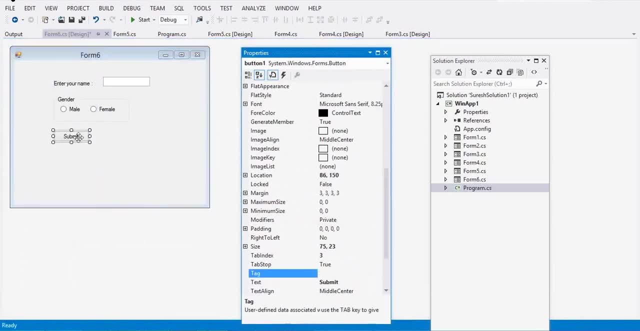 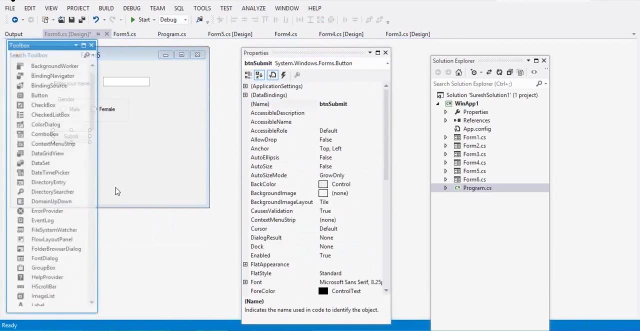 I'm telling you to proceed, or you can say: submit whatever you want. So here I'm, taking this obedient subject. Now, what is my question is, when I click on this, I want to get the status into my text box label. 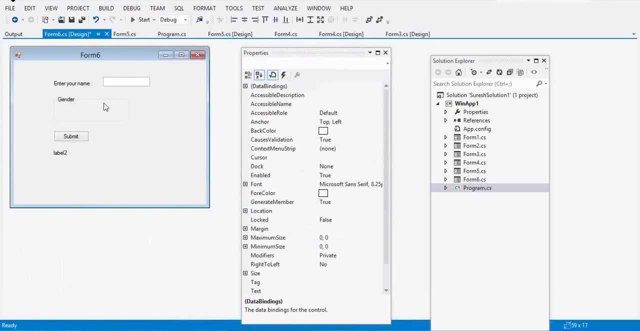 So this is my thing. what I'm going to do is I'll just put it in the corner. okay, control X. okay, keep that there very clear. Now, what is my question is: when I click, I want to say welcome, Mr. if you select a, 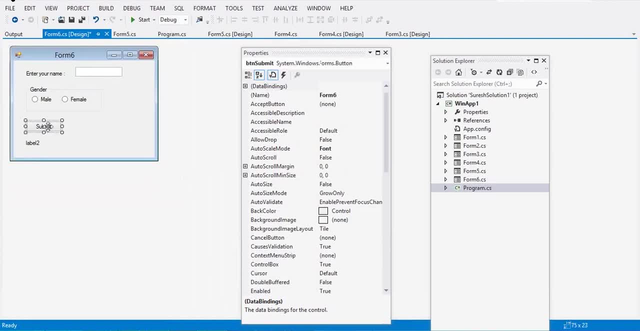 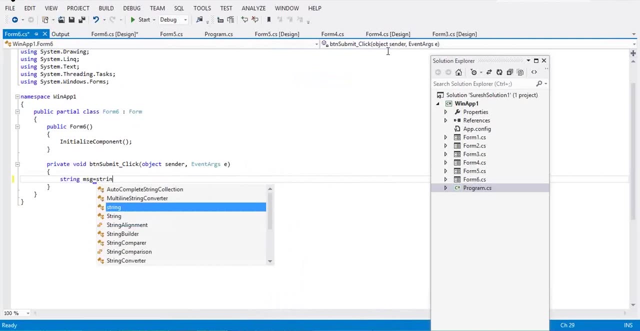 male if you click on the female. I want to say: welcome this. let's say this here. I'm going to say this String message is equal to string dot empty. it is strongly wanted to have empty when you don't have any data. 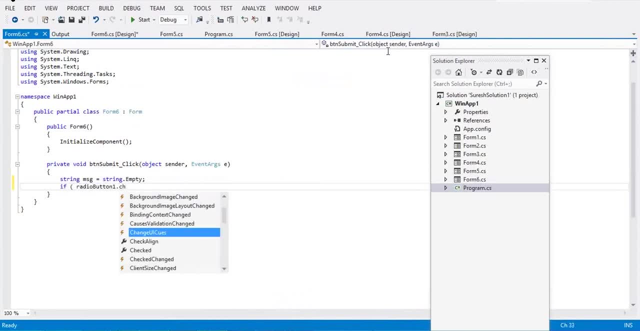 Here I'm writing X radio button 1 dot check. So what do you mean by radio button 1 dot check, For example? if you say the first one, then I'm writing: message box is equal to okay. here I'm writing something called welcome, Mr. 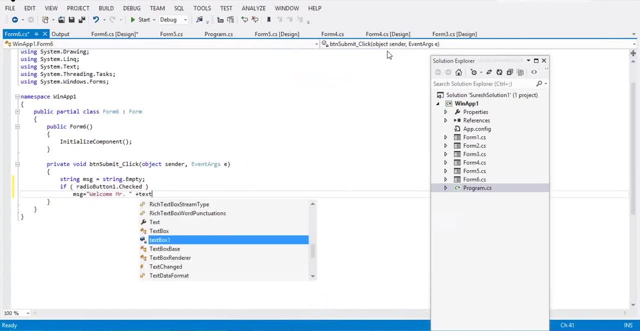 Followed by text box: 1 dot text, For example, I'll say: radio button. 2 dot check. Okay, same thing. Message is equal to welcome Mrs Or Mrs, Whatever you feel comfortable you can say Text. Finally, label 1 dot. 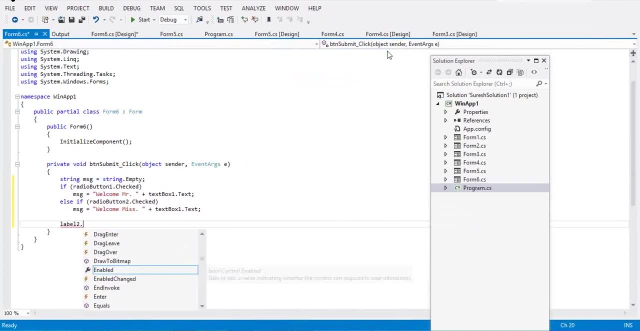 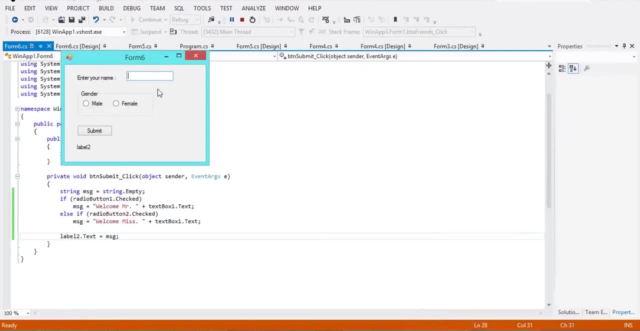 Okay, wait. 2.. Same text box Label: 1 dot Text is equal to MS. Let's execute this Okay, Here, Here. Okay, Now Take on a male, I'll take it. Welcome, Mr Okay. 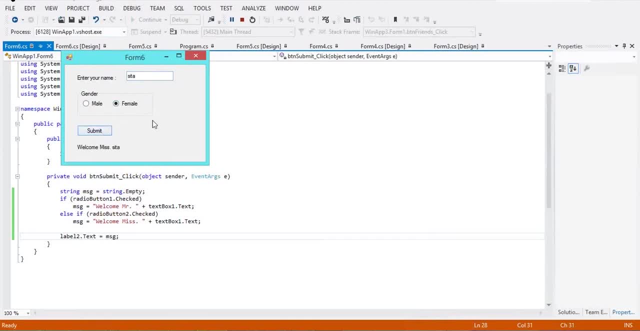 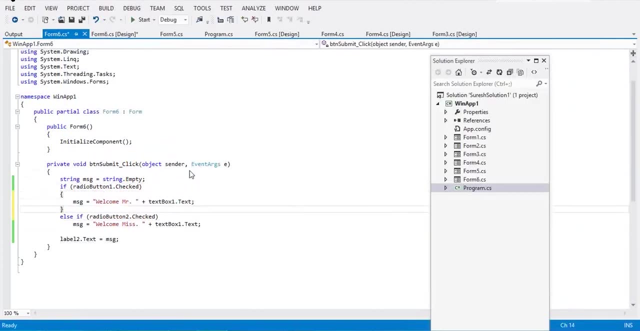 For example, I'm sending something called Sita Sita. Okay, I'll miss it. Okay, No, no, Let this. I can do some programming also. Let's say this: If you send it, Okay, If you send this. 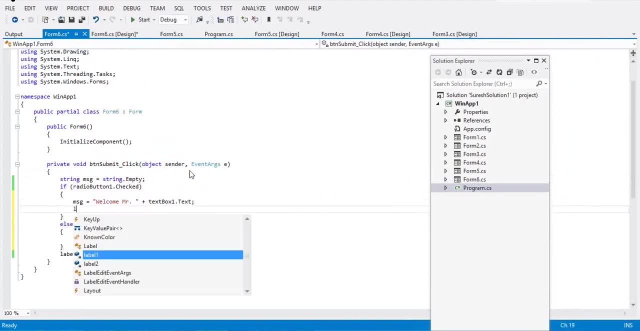 What do you want? For example, if I send it a male, I want to say: label 1 dot, label 2 dot. four colors here: Color dot, Green. For example, if I send this: Label 2 dot. 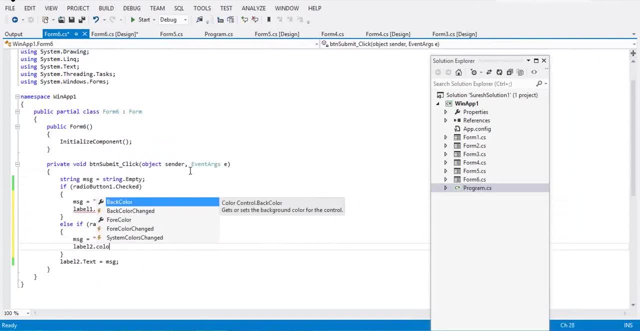 Color is equal to blue. Four colors equal to color: dot blue. Let's execute this. Okay. Here I have given something called Okay, This is a female. Female is coming on. You can. This is a male, It's coming on. 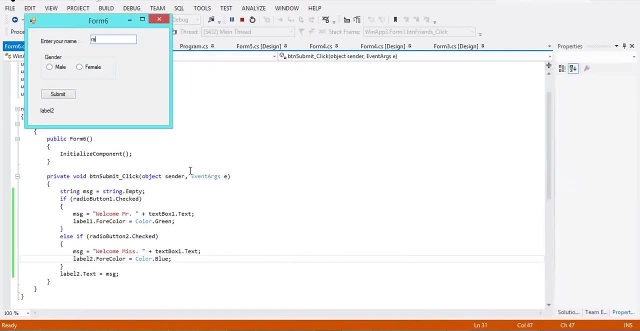 Both are coming. See, I wrote something wrong here. Green, I wrote green, So we need to go for the label 2.. Okay, I was mistaken. Let's execute this Label 2. dot Color is equal to blue. 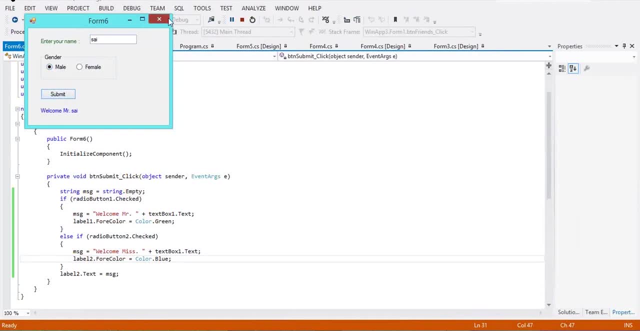 Four colors equal to blue. Color dot Blue. Let's execute this, Okay. Here I have given something called Color is equal to blue. Let's execute this. Okay, It's a blue. Select it. Google Select it. 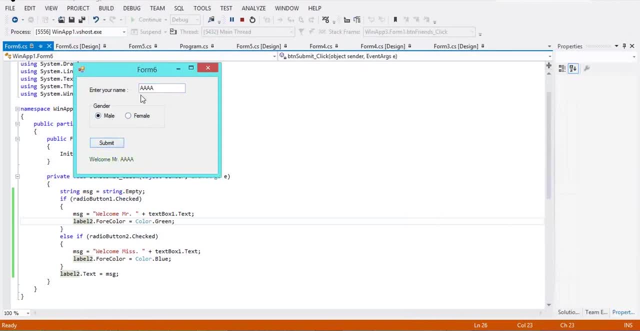 I can do it. I can do it In water, So any manifestations you miss or misses are changing. You can, Okay, So this is what exactly? If you are able to see this. I have some more examples on. 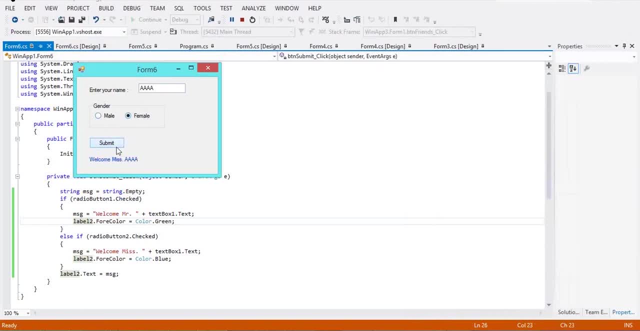 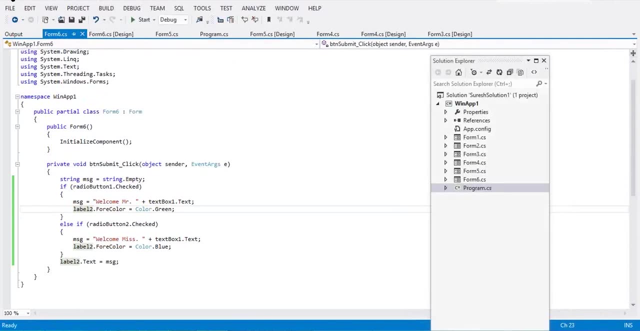 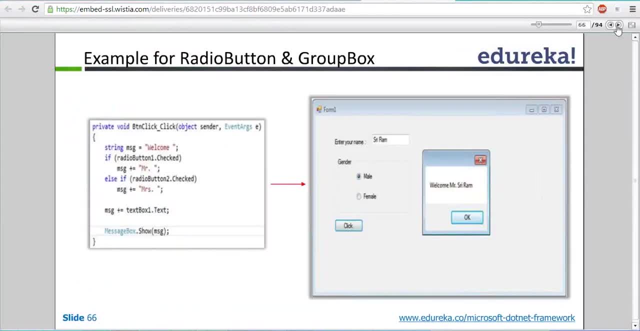 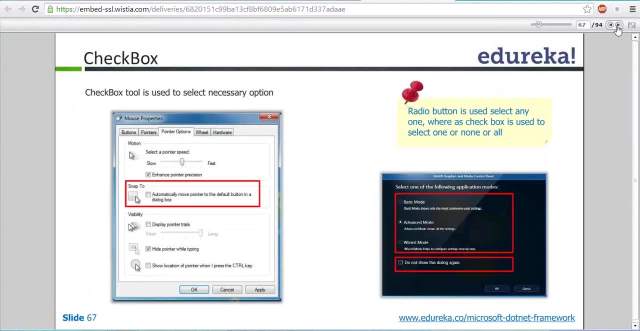 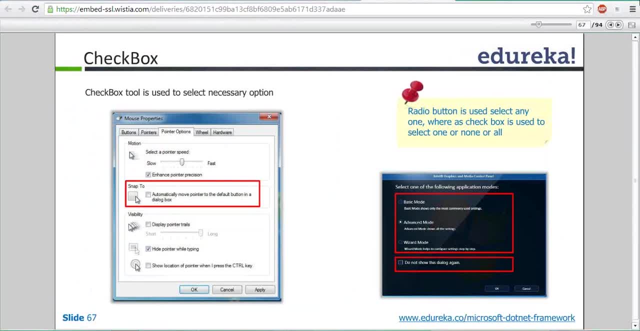 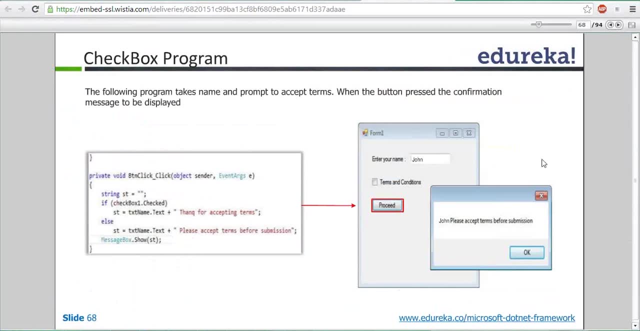 Check box is used to select one. Radio button is used to select anyone, whereas check box is used to select one or none, or one. See this: here I have a name and I'm asking you to please select terms and conditions. If you click on proceed button, I'm telling you that. 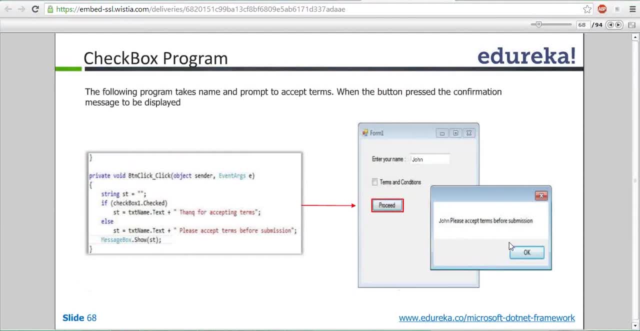 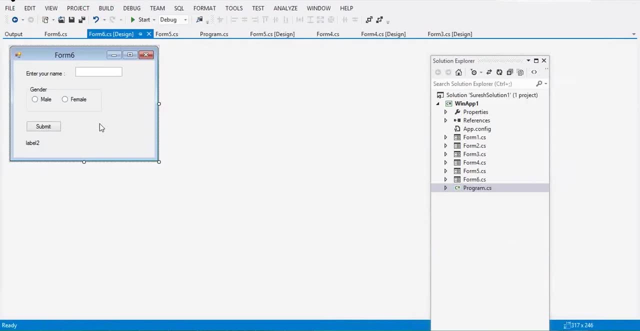 If you select thank you message to be given. if you don't select, I want to give you. please select. Let me see the same example. Let's see this. I have a form Here. after giving this, I would like to have a button called check box. 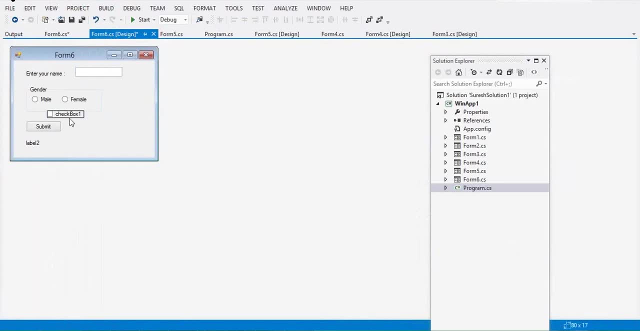 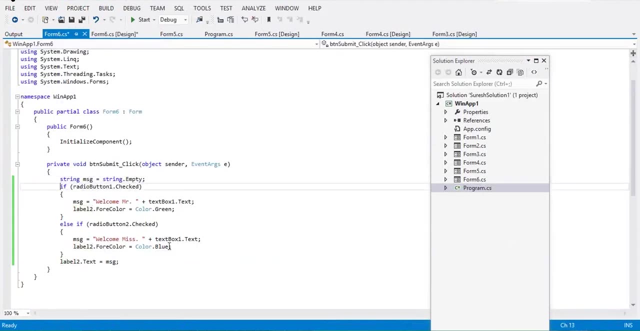 Let's say this check box: So this check box to be displayed before submission. and here I'm asking you to change this. Let's see this Here: if radio button is checked, Here I'm writing: let's see this: remove this radio button code. here I'm writing. 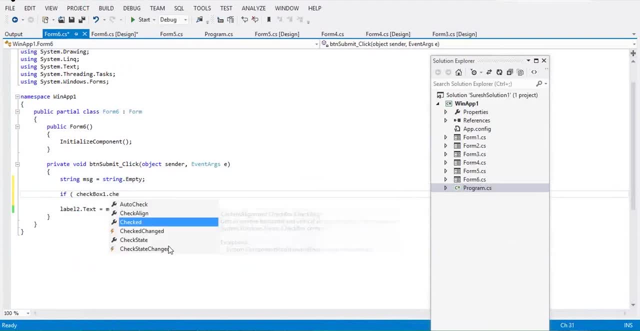 If check box will not check, that indicates if you select this. so here I'm writing: message is equal to text box will not text followed by okay. here I'm writing: thank you for accepting terms, Terms Else. here I'm writing: message is equal to okay. text box will not text: okay here. 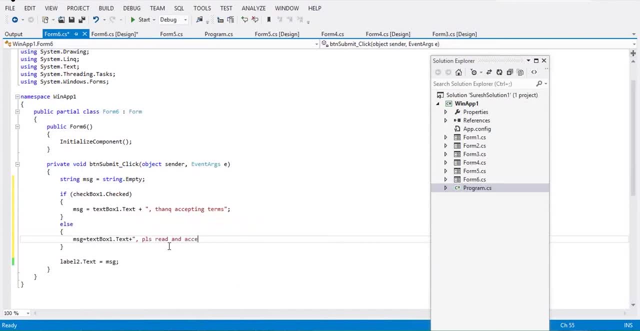 I'm writing. please read and accept So here. if you're okay, then fine, label two dot text is equal to green color. If you accept the terms, very good, I'm happy. so I'm giving label: label two dot, four color. 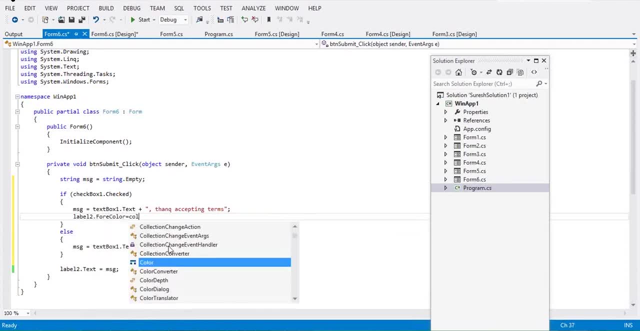 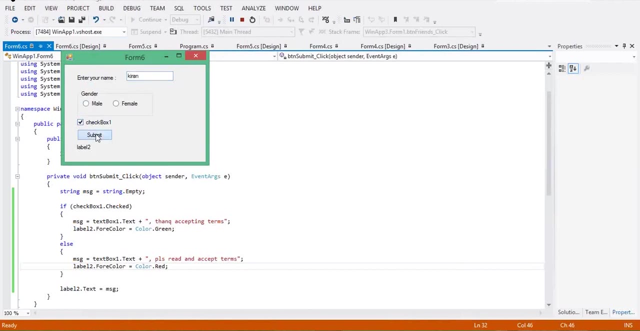 is equal to green color, Correct, For example, if you don't select it, I want to give this one label: two dot, okay. four color is equal to color dot red. See, like this It's correct. Okay, I selected the terms, so it's telling. thank you for accepting the terms. 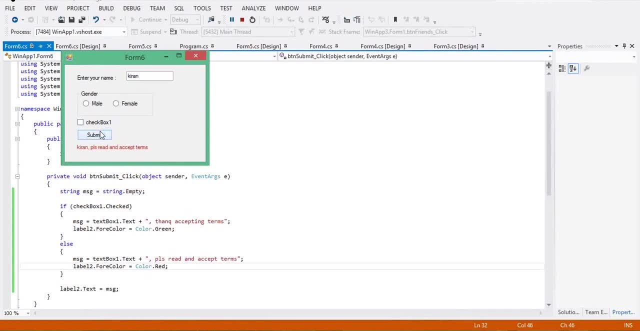 For example, if I don't select, please read and accept the terms. See, this is a very, very easy. while working with NET it's a very, very easy, okay, but it's very, very important in the real-time scenarios. 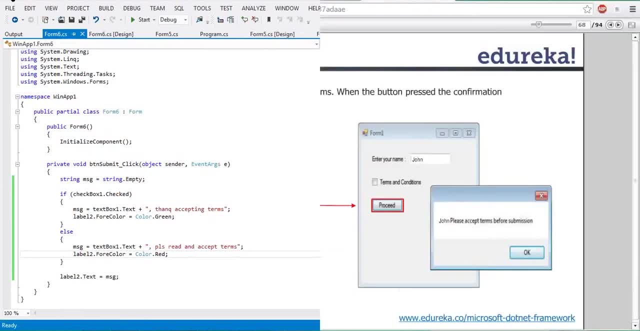 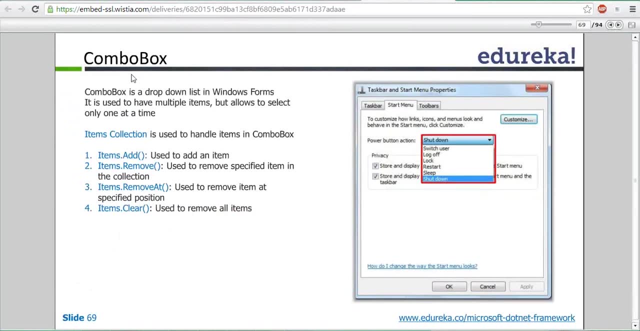 Okay, Let's see the same examples here. okay, check boxes we have seen Coming to the next one. okay, So we have something called combo box. What is a combo box? Combo box is a drop-down list. Combo box is a drop-down list. 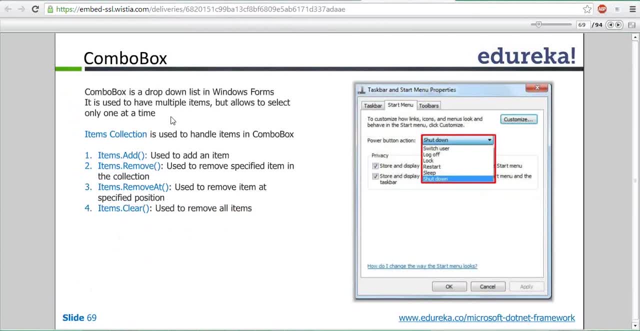 Okay, It is used to have multiple items, but allows to select any one. Okay, How the combo box is going to be working Internally. there is something called as items collection will be there. What is collection? Items collection. So this collection helps you to handle it. 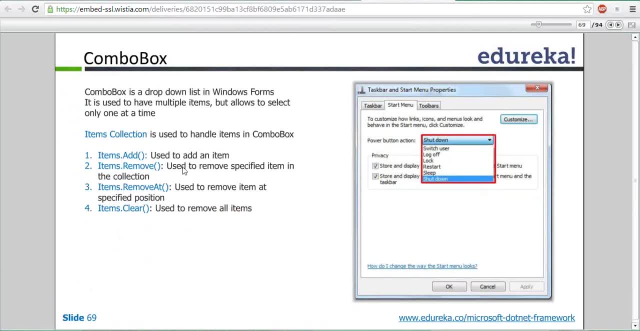 For example, if you want to add an element, items dot add. If you want to remove, items dot remove. If you want to remove on items dot clear, Okay, If you want to say something, it's what are going to be. 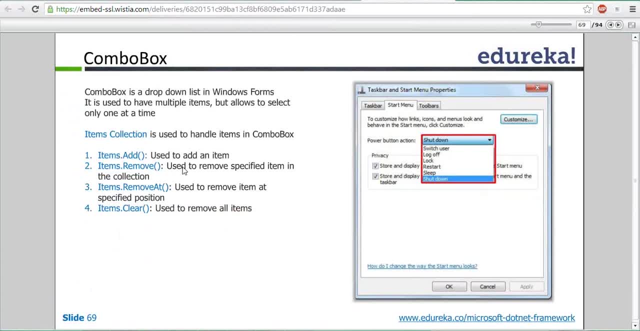 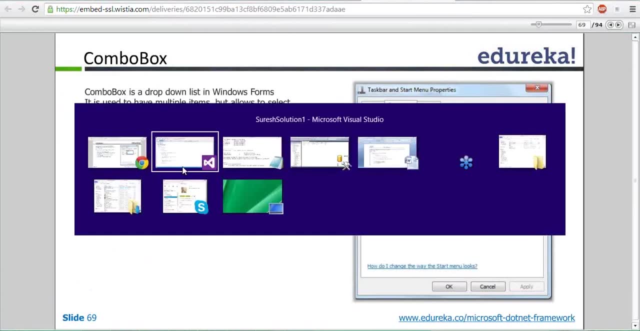 have an related to anything will be done using this items collection. Okay, So how an items collection will work. Well see. Okay. Let's see an example from tactical. Okay, I will be adding one more form. I click on it. 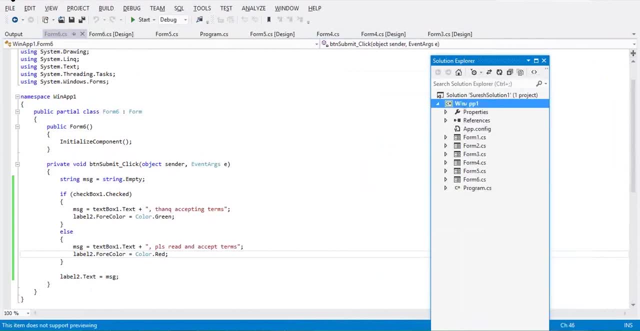 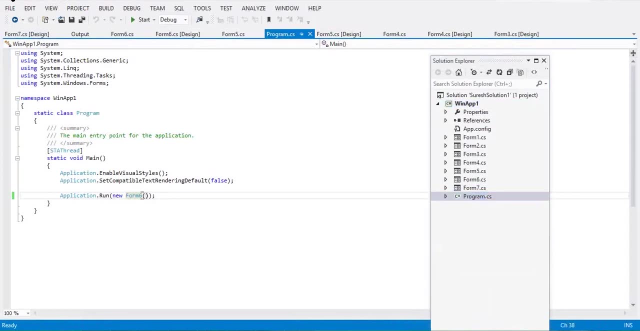 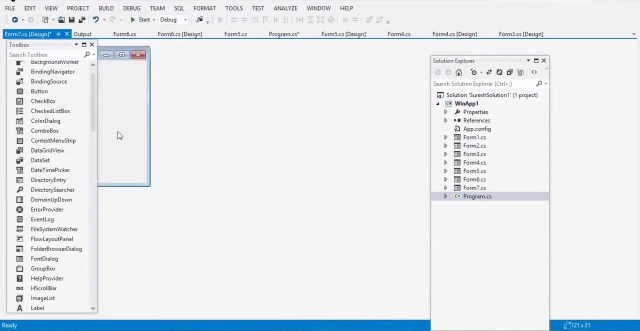 Add: Okay, And I'll change this one to 7.. Okay, Okay now let's see this here. I want to have a common box, so this is common. let's see this. I will be having a common box by default. there is nothing. okay, see that. and the style. 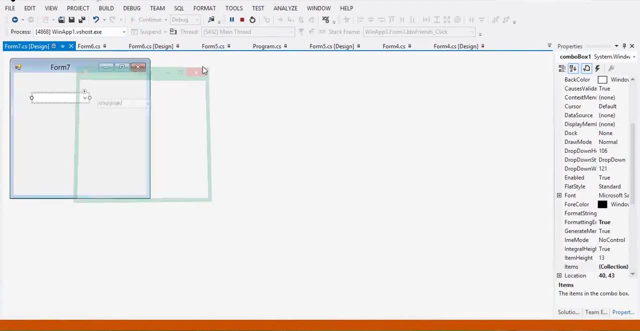 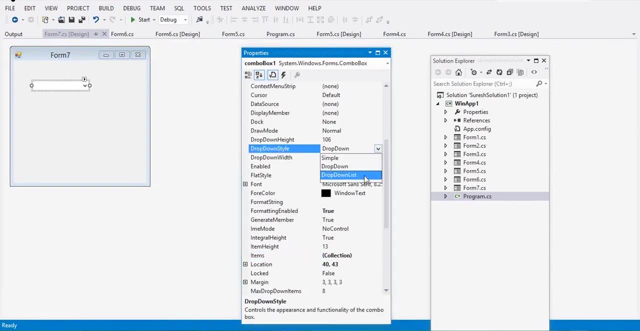 is allowing to type it. if you don't want to allow to type, change the drop down style. there is a property called drop down style. okay, so drop down style. change the property to drop down list. so what is drop down list? it will not allow you to type. let's exclude. 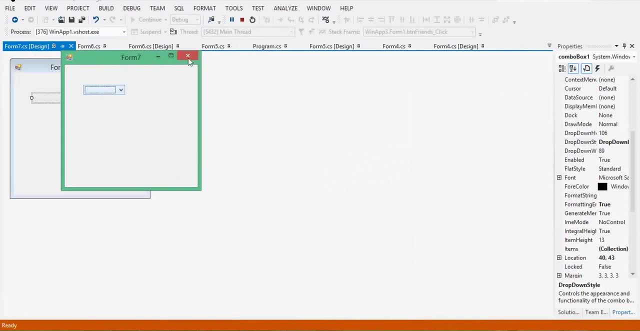 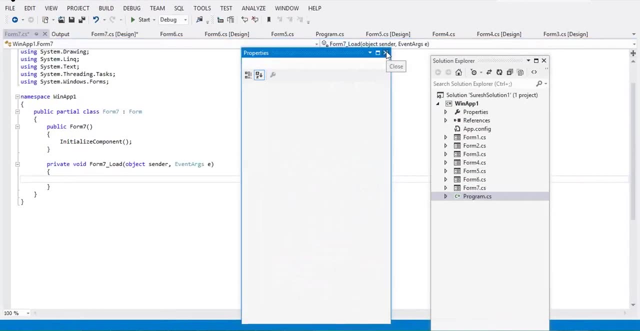 it. it will not allow you to type just simply if you want to have something you want to copy. it's simple what we need to do. there are many ways: combo box, window items, dot. add what do you want to add something that not like this? you can add something now. 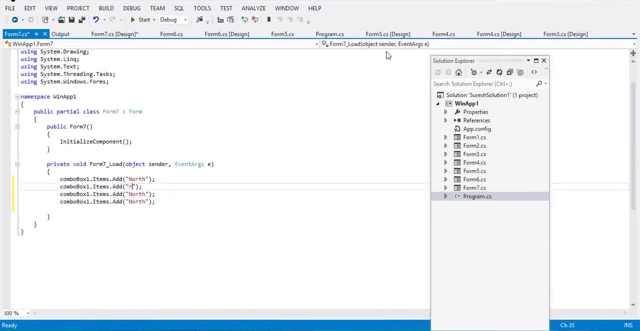 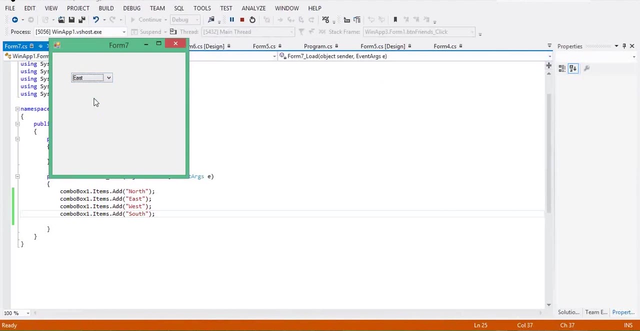 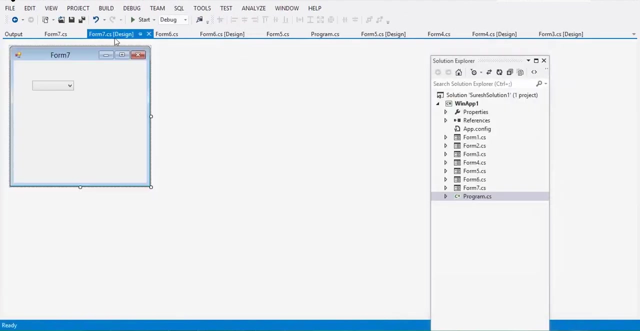 what happens? four items are added for you. okay list, okay list, let's execute. let's do that. simply see. and again, for example, when I select something I want to do, simple, never mind, what do you want to do? I want to say something called I will put a label. 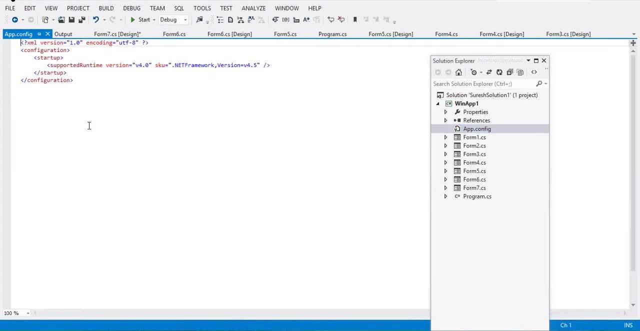 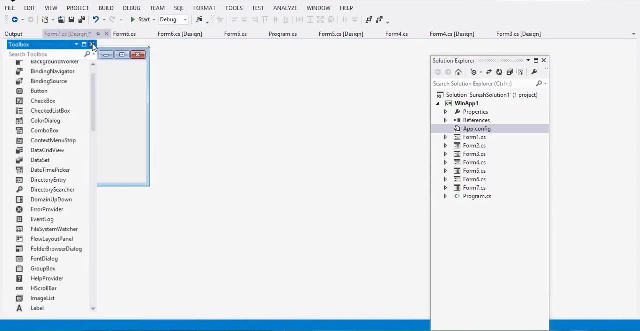 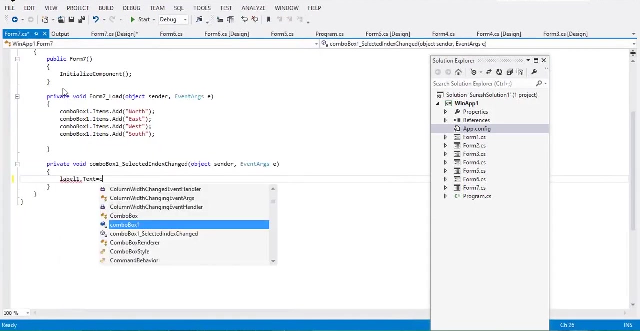 first of all. so I have a label. so what is that label here? I took a label here and when I click on this, yeah, I'm ready. level1.text is equal to combobox1.text, so let's execute it. keep on selecting this. 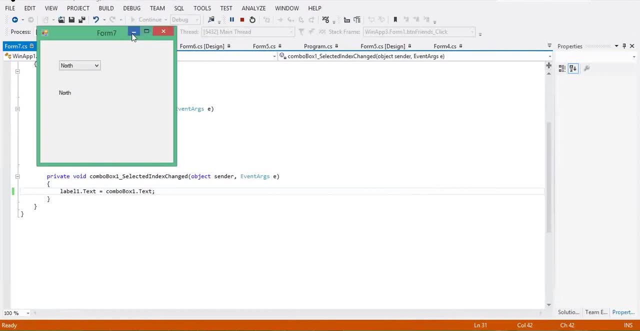 keep on applying. see how simple. it is very easy. see if you are able to see this simple. it's very easy, straight away examples. very, very easy to do things and you will be also getting some exercises also. you can see them. it's very easy. see how simple it is. combobox. 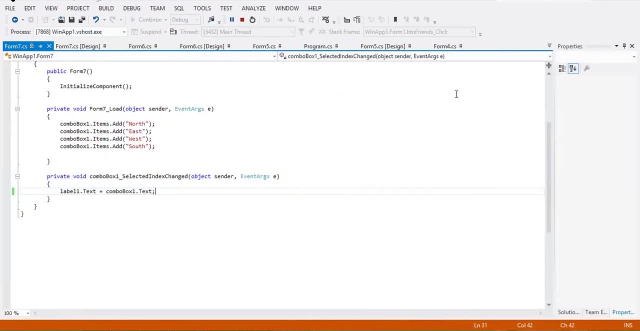 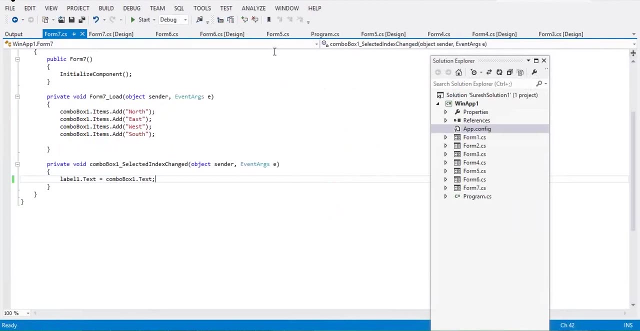 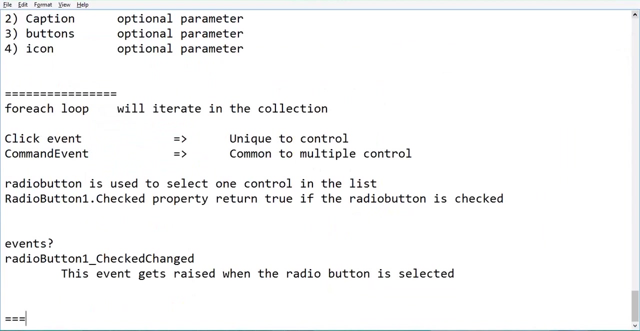 see similar to this combobox, we have something called listbox. combobox allows you to select any one, whereas listbox allows you to display multiple options. so in order to work with combobox and listbox- both are same, so combobox and listbox are list controls. was that question? 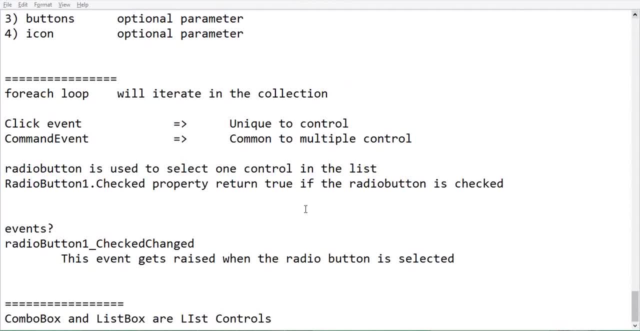 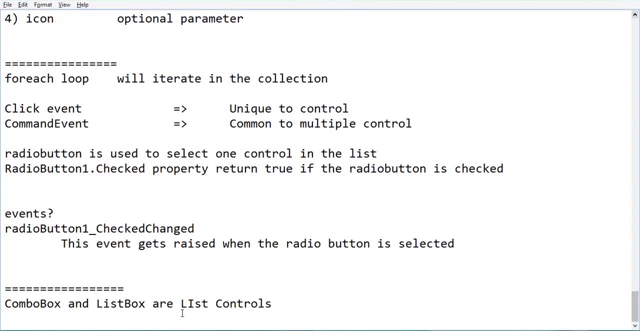 what does link mean? why do we need it just before anything? sure, we will discuss the link before winding up the session now. combobox and list controls are both same, so used to have multiple items. combobox is used to select single item in the list, so combobox is used. 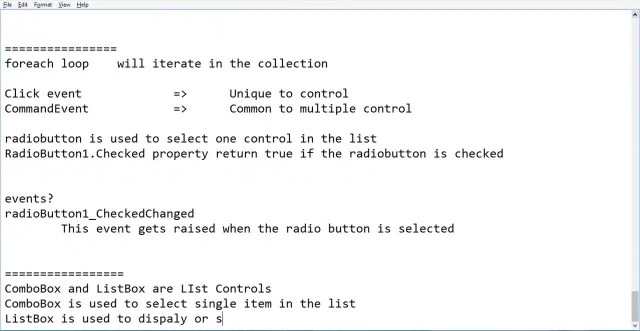 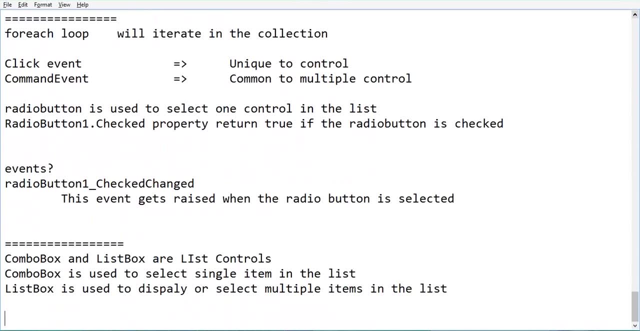 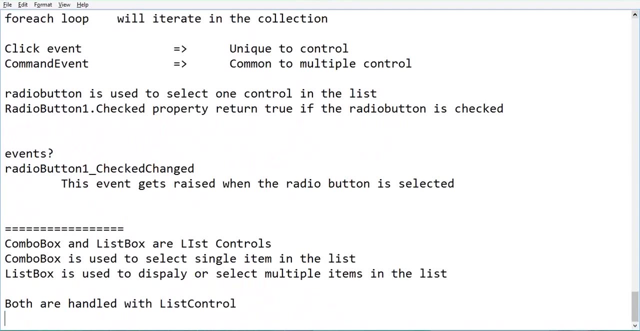 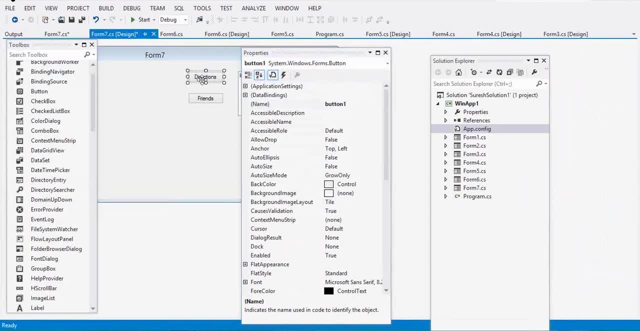 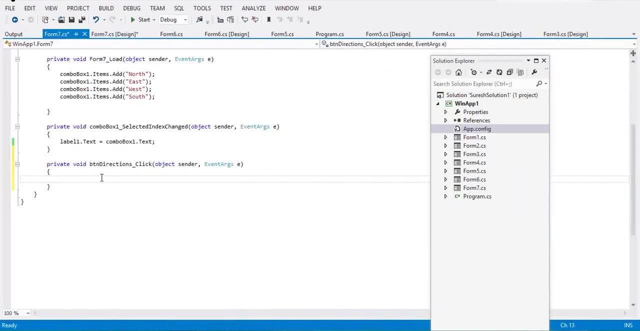 So let's take on it. so here, one of the directions is simple. you can declare a string at it, which we discussed in the last lesson. string directions. I can say directions is equal to. I can say not list, list, sub. if you want to display this, I can simply say that listbox. 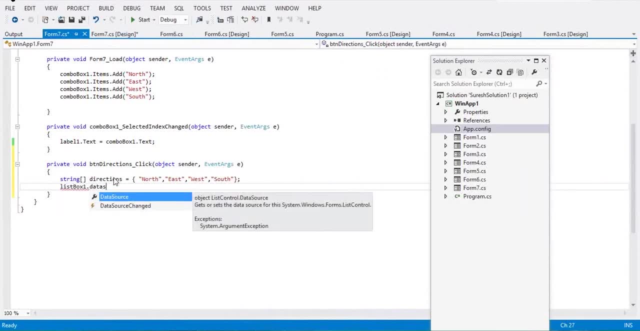 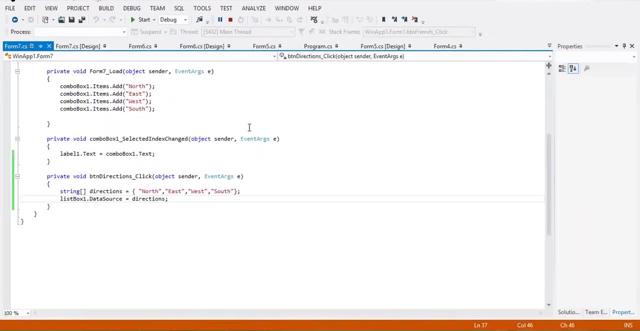 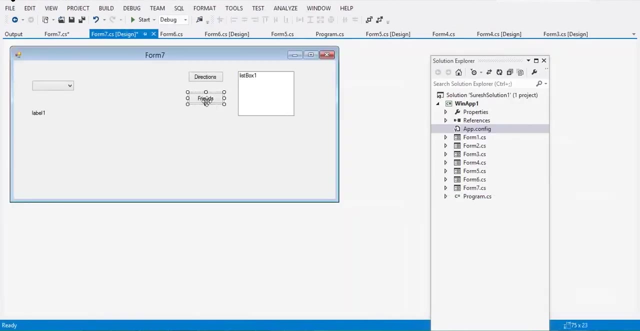 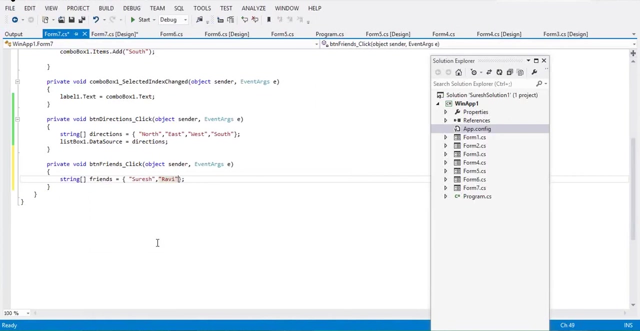 one dot data source. there is a property directly data source in good directions. let's click on it. now let's come to the second one: friends. here I can say string friends is equal. so I can say: service. okay, company car break, okay, update. and here I can say service. 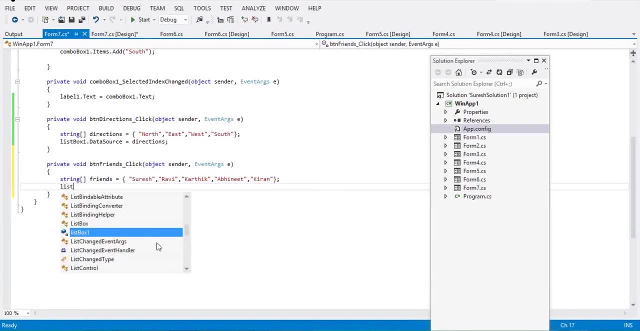 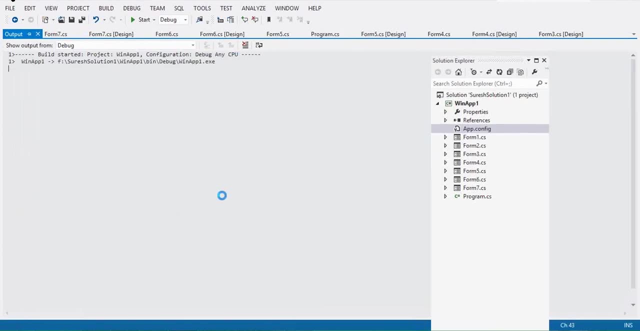 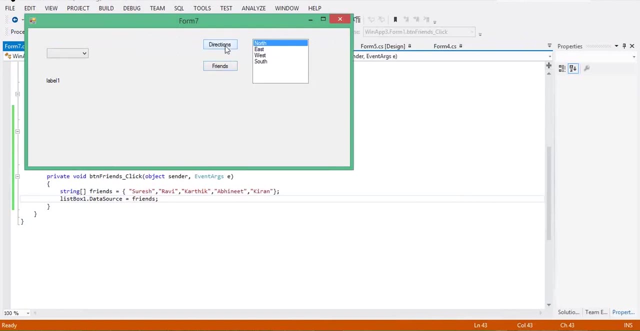 I want to add this simple listbox: one dot. okay. data source is equal to friends. it's possible. let's say this: credit directions, get it. see how simple it is. multiple items are done. okay, we'll see one more. a real-time example how simple it is. we'll see a real-time. 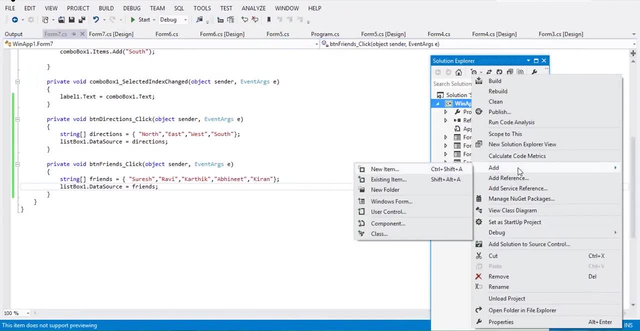 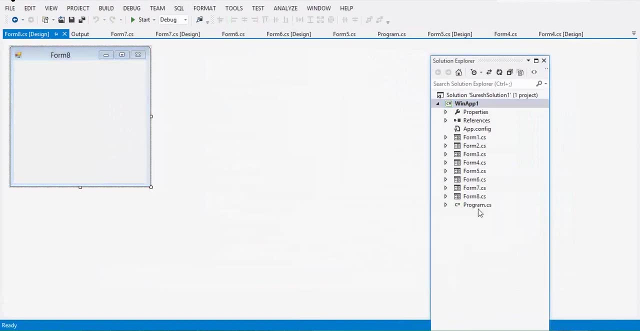 example, which I wrote for one application- see here One form. I can say this: the form is eight. okay, now I'm using this, it's eight. let's copy this here. there's something about this label here. what I'm doing is I'm adding some. 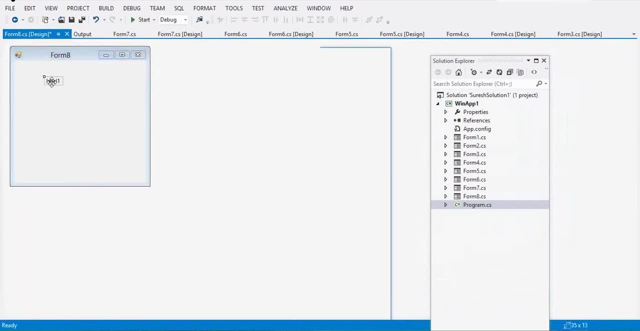 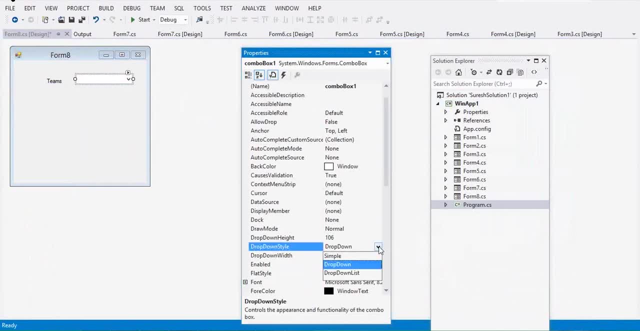 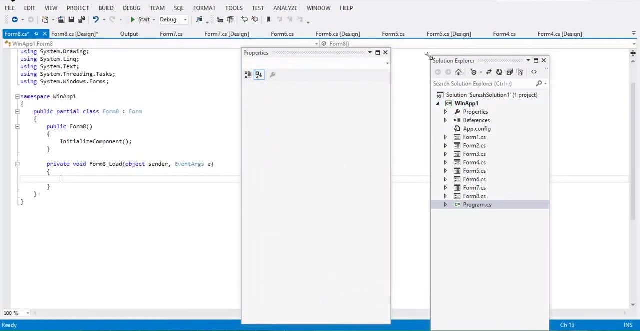 list equal to drop-down, so that nobody can change. So what are the things which are required? So here, what I'm writing is- it's a real-time example which I wrote for all applications. I'm writing teams. I have some teams like this. what are the teams? administration team. 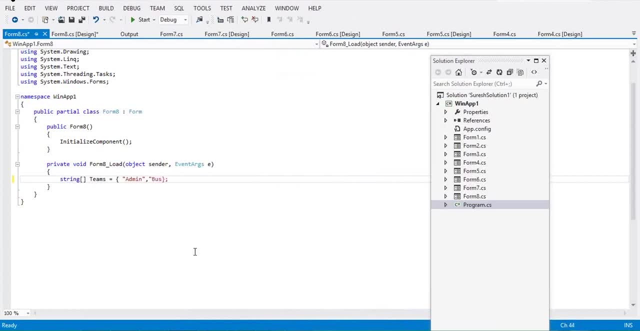 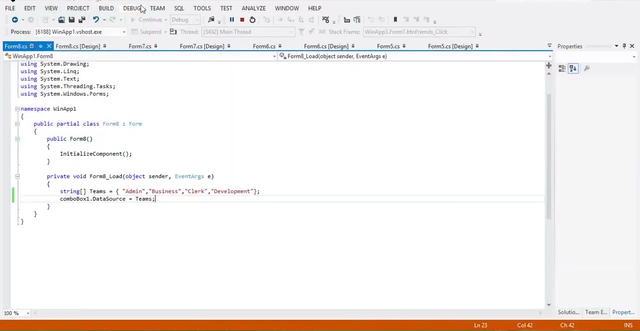 okay, I have something called business team. okay, I have something called. I have something like this: this is so. what I am doing is when I click on this. okay, so colmovox1.datasource is equal to this. let's see this. when I exclude this, I am not supposed to select anything. 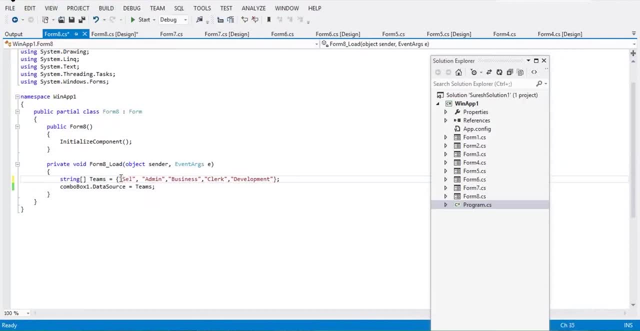 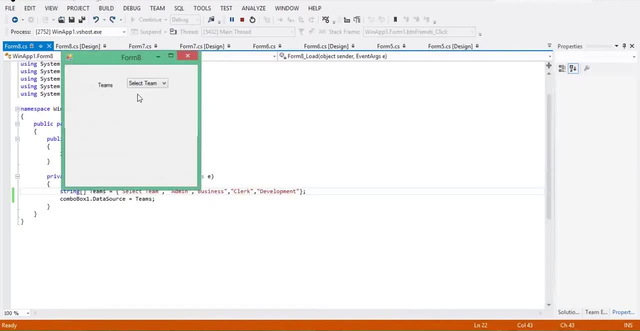 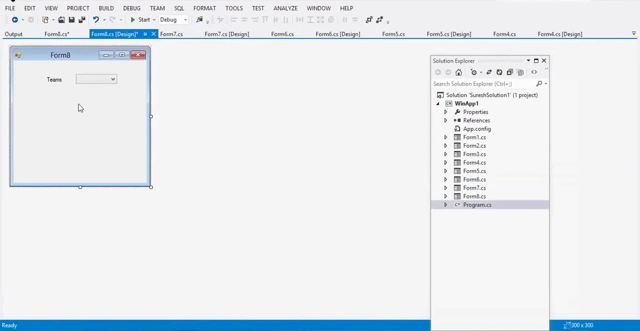 so initially, what I am doing is I am selecting this. let's exclude this. now, what is my question is, when I click on a particular team, okay, the team related team members to be displayed. so I am using the list box. so the list box should contain the teams. what teams I want? 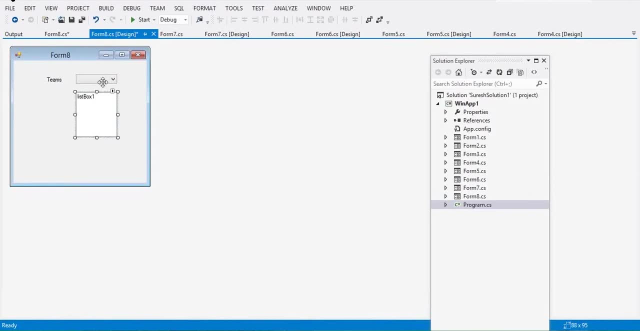 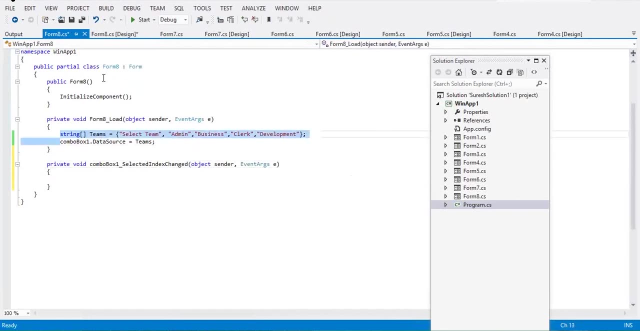 to display. the selected team should be displayed. the selected members. let's say this: how do I do this? Let's say this one: here. I will be having list of the teams separately, so better take them as a global variable so that everybody can utilize this. so I have string, okay. 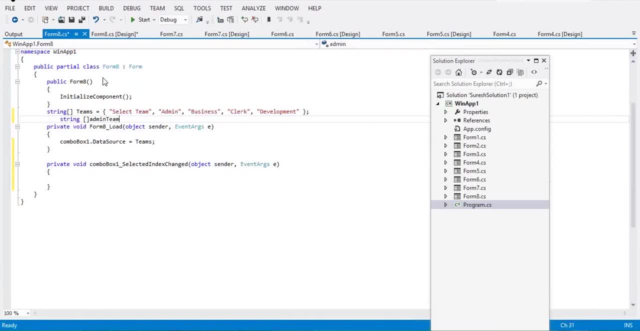 I have something called so I can say, okay, so variable name should be always okay, so I will use this. okay, so is equal to see here. I will have this number file for my reference purpose. I am giving copy, but this trend in business is equal to here. 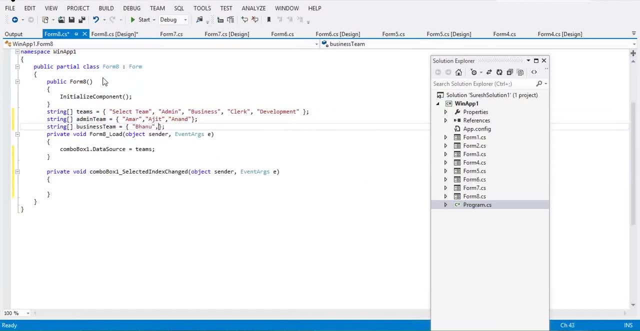 I can see. so I am giving different number also, so that it will be very clear. next one: so only one candidate is there. I can say so. this trend in development is very clear. so I can say so. this trend in development is equal to W Z quad. so I can say this. so. 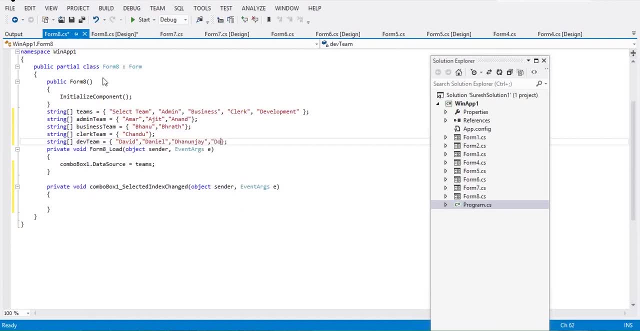 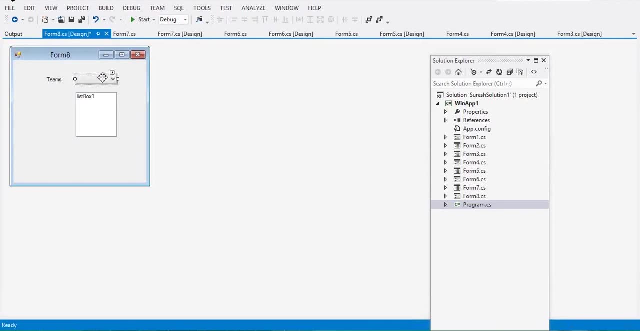 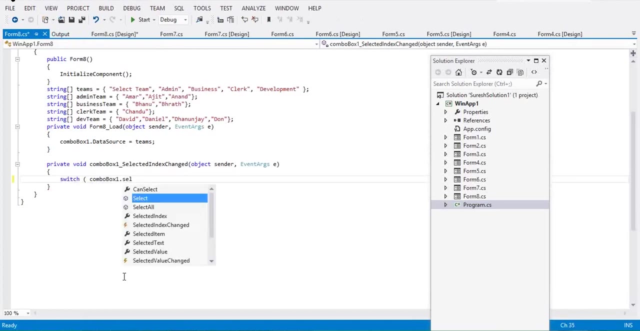 for my reference I am giving like this. Now, what is my question is, when my list is changed, list box to be changed. how switch case? what is the switch case? combo box 1, dot X, not select an index. See, the thing is also very easy to understand: Select an index in. 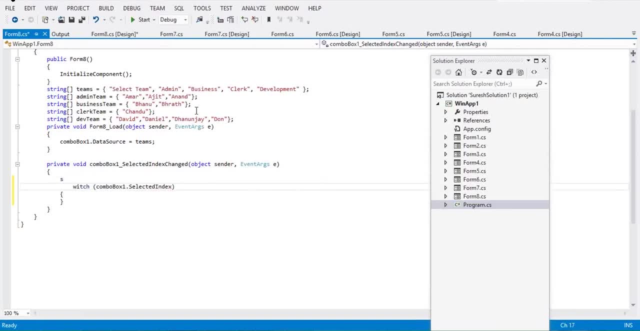 this instance, which position have been selected. If you select anything under 0, nothing should be happening. If you select 0, nothing should be happening. So k is 0.. What do we need to do? Nothing. So list box 1, dot data source is equal to 0. Nothing should be there For. 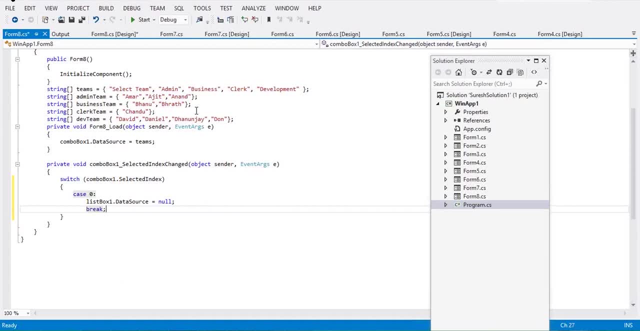 example, if you select 1, what is 1?? I would like to have admin name. List box 1 dot. I would like to have admin name. This: Okay, Say case 2, list box 1 dot. data source is: 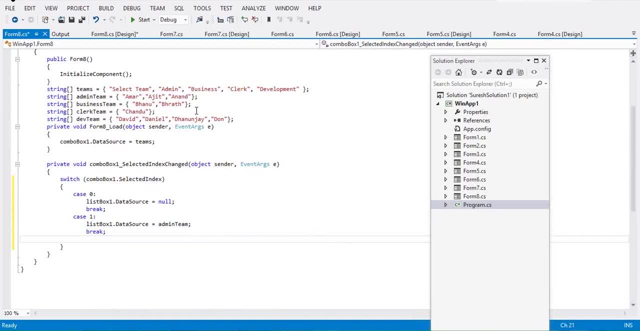 equal to something called business team. Same example: Break Case 3, list box 1 dot data source is equal to break Case 4, I can say that list box 1 dot data source is equal to something called business team. So you can understand that whatever you select, it will. 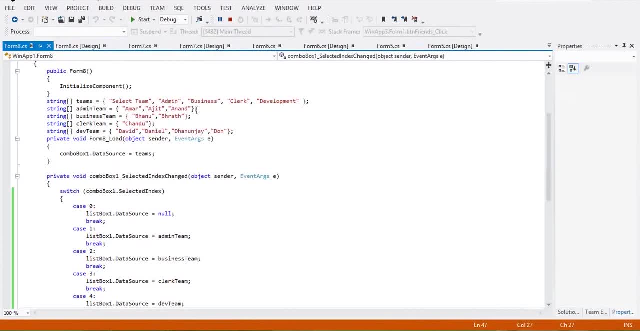 be. Let's say: this is correct. See, I'm selecting. See, I'm selecting. See, Let's change this one to something else. See, Whatever I'm selecting. the rest of the things are coming. Am I clear? 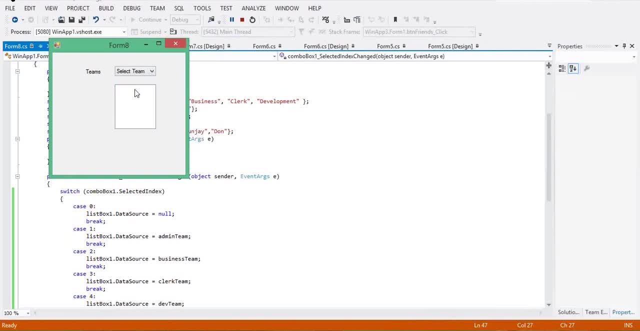 So this is very easy. Real time scenarios will be like this: See doing the Windows applications or doing the ASP applications. you don't even believe me. We can complete your applications in the map In a matter of minutes, not even in a matter of hours. also, Small, small applications: we 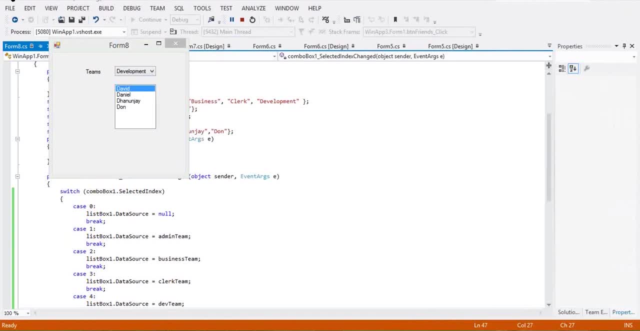 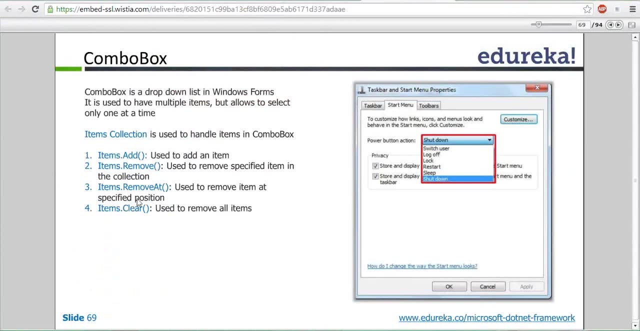 can do it. Okay, This is the easiest way where you can do it. Let's see the content. So what else we have? We can see this Como box I send you that You can use: add, remove, remove it, click Okay. Let's see this next example. Selected index. We have the selected. 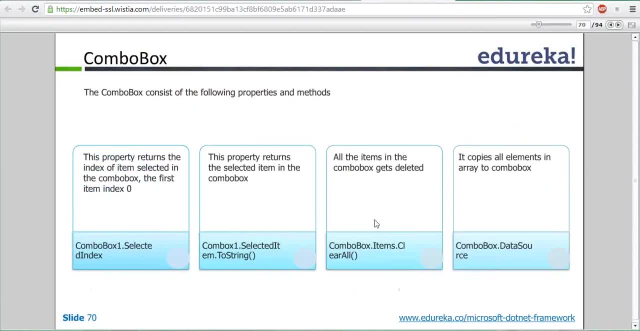 value: Selected item. We have the item which was selected: Clear Clear all items. gets clear Data source. Reference to the all items. Copy this: All right. How to select items. Here I have an example. I have some products. 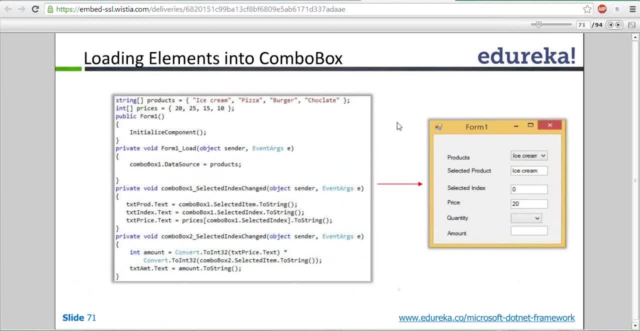 which was there, like ice cream, chocolate, pizza, etc. When I click on any item, the item to be displayed, item index to be displayed And item to be priced, price to be displayed. And when I click on the quantity, the rate of it to be displayed, Amount to be displayed. 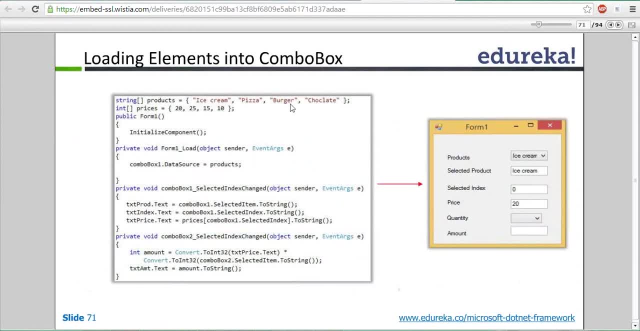 Let's take this example, How we look at it. So products are there in array And the respective. When the form is loaded, I load the products into my drop down list. When the combo box 1 is selected, it changes. 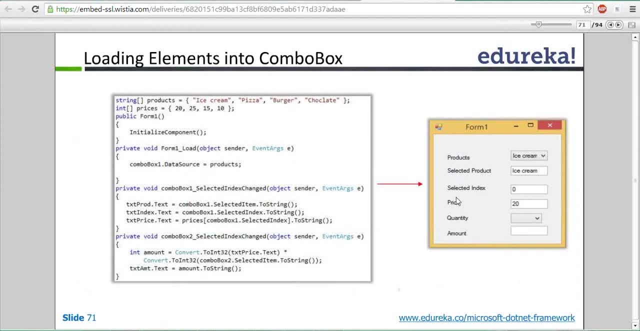 If you do any changes. in the combo box 1, I'm giving txt product. In the second line, I'm giving the item module selected. In the third line I'm giving the index. Fourth line, I'm displaying the price. 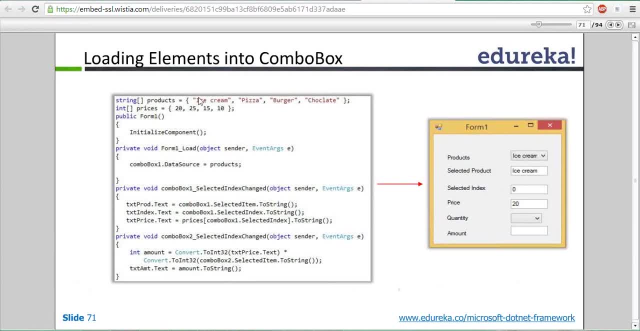 Price is here. As I said earlier, item is 20, pizza is 21.. So these two are matching in the same place. Now I'm doing the same thing: Pricetxt equal to pricecomo1.selected. So whatever you select, pricecomo1.select- 20 will come, pizzacomo1.select- 25 will come. 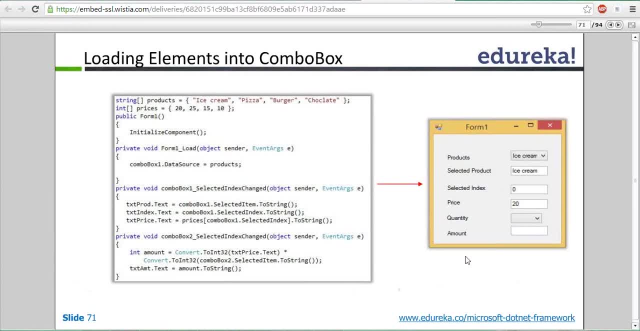 And what about the second one? which one? your combo box 2 is changed. What I'm trying to do? you'll be getting the quantity, So find out the amount. Amount is equal to txt price which we are getting from here. 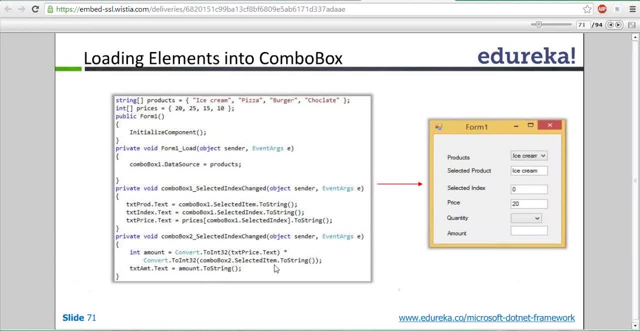 And quantity is equal to what. So in here I was going to say: okay, price into quantity, price into quantity is coming from this one. So price into quantity, into whatever is in between, Okay, It's the same thing. Example what we have. 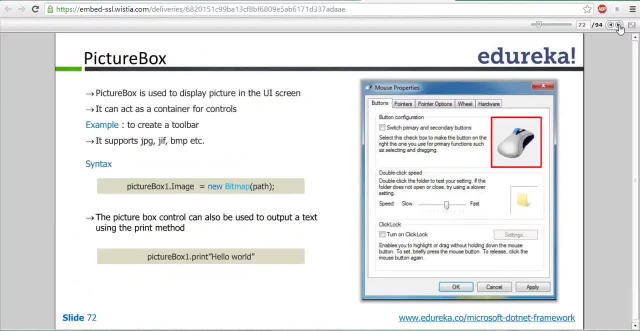 Right Next. So picture box: you can get some picture boxes. How to get a picture box? Very simple Picture box. you need to drag it Picture box on that image equal to new bitmap and any path. Let's see this example. 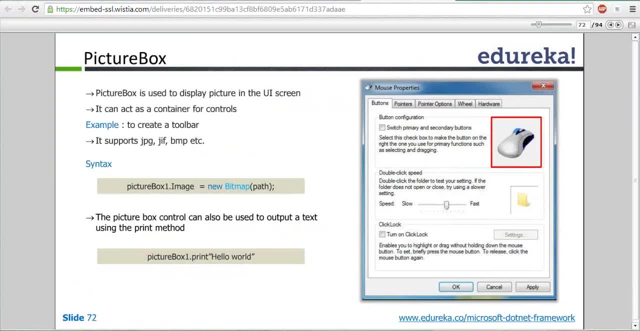 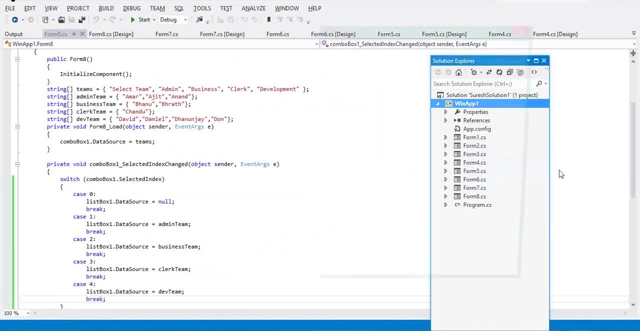 And practically So. this is also very, very important here. Very easily, you can develop applications. Let's see a small example. Add, Okay, Windows forms. I have a form. Okay, I would like to have a picture box. So this is my picture box. 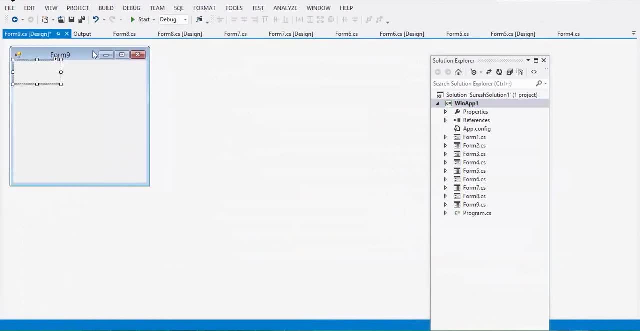 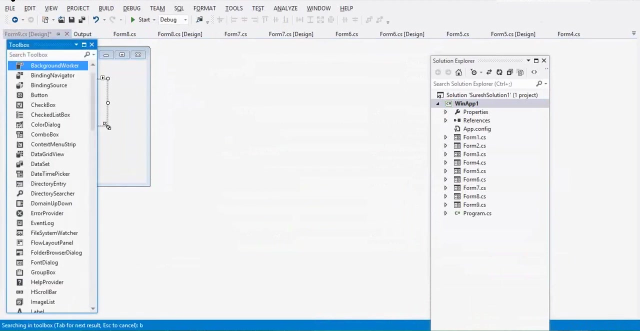 My picture box is So. you have size modes on there. Please change the size more to something else. I'll change this one to stretch. Okay, So I can have a stretch which is One picture box. For example, I would like to have a button. 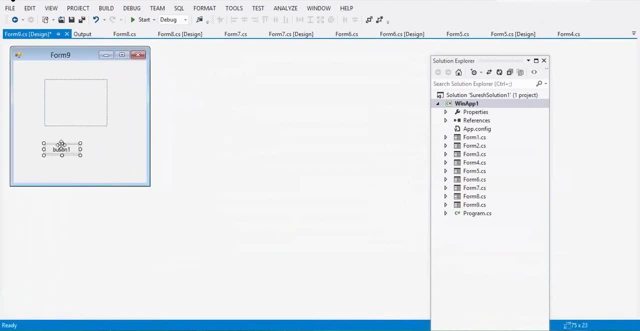 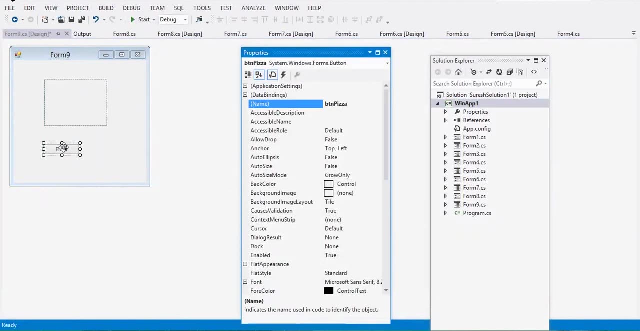 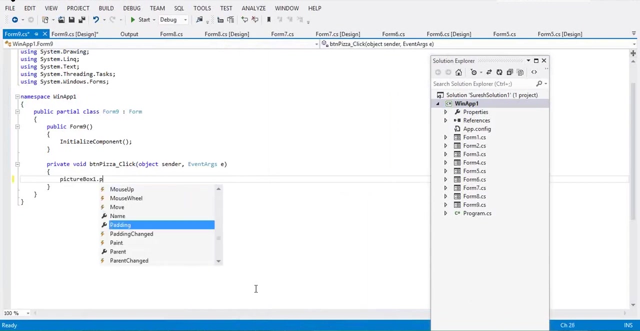 One-handed click on the button. I would like to have something called as a burger or pizza Pizza. Okay, I have the collection of items in my C drive, so I'm going to picture box. one dot picture or image is equal to, and it's a new bitmap. bitmap is a place where we can store the data. 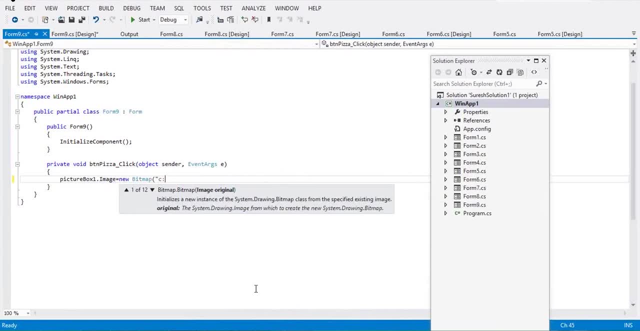 It is available in somewhere. Actually, you need to do the path C column. I have it there in my full images. Okay, These are jpg. I have it jpg Now. when you write this program, it will not understand what is this. 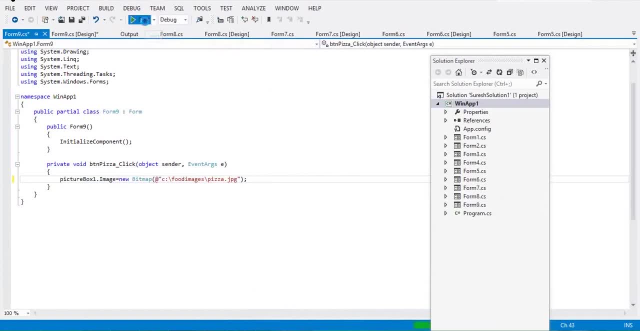 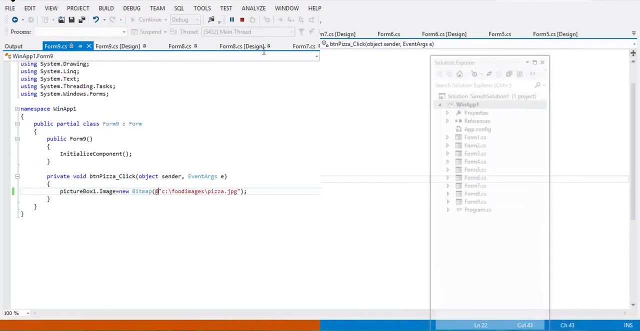 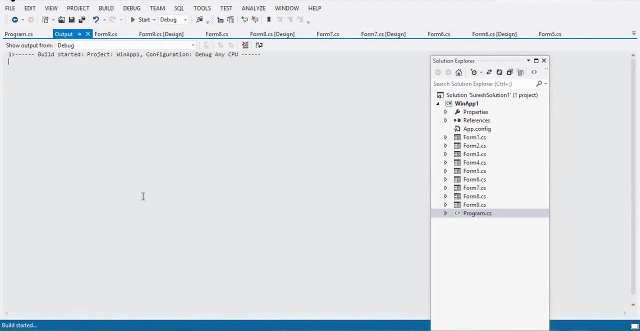 So put that, Let's call this, Let's click on it. All it is running right. So what you need to do is open this, Make your application start up as Let's open it. I have the images in my. 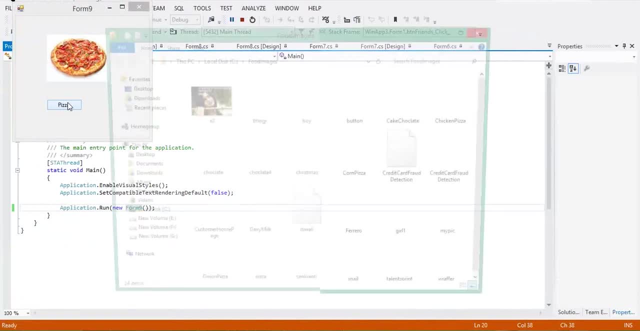 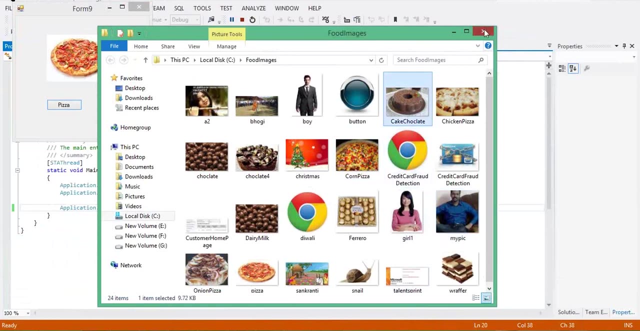 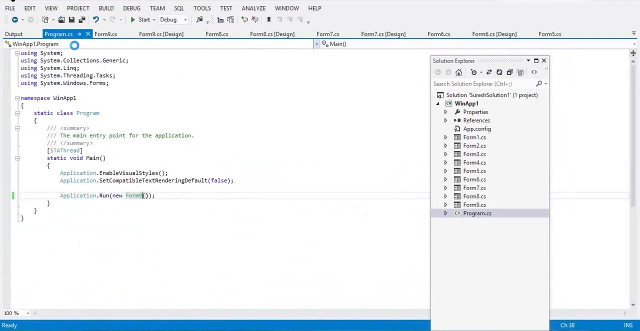 So all these are, All these are. I can print my picture, I can print my, For example, I want to print my picture, Okay, So what I'll do is I'll add one. Okay, I'll add one image here. 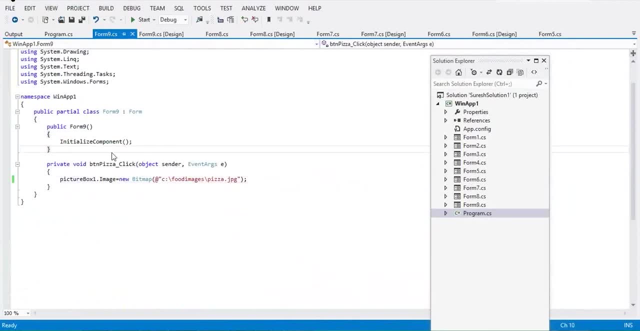 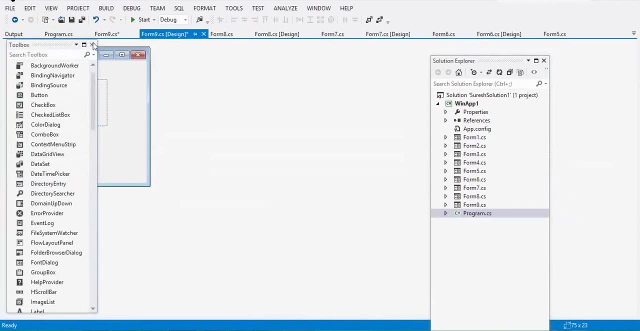 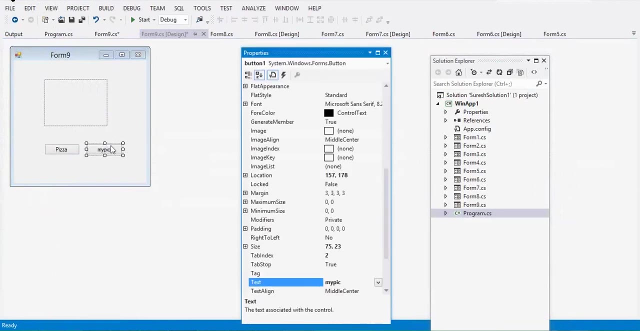 Okay, So Okay, I'll. So I want to display my pic, Okay, My pic. So I have to look at. I'll change that Picture box. one dot image is equal to So same thing. 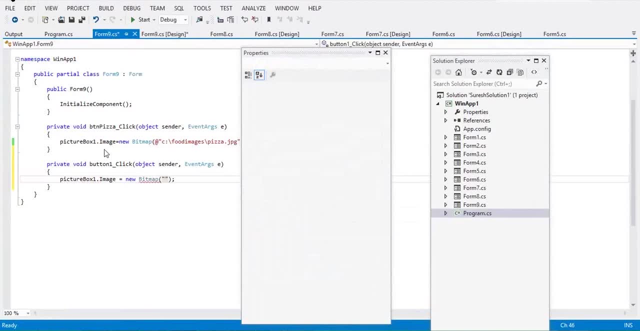 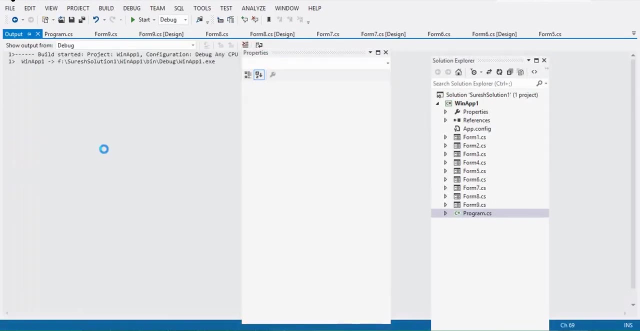 Okay. So here And there is. I give them my images. Put images, Okay, My pic jpg, So I can. That is correct, Are we getting this? Yes, Let's Okay. Any easiest way is. 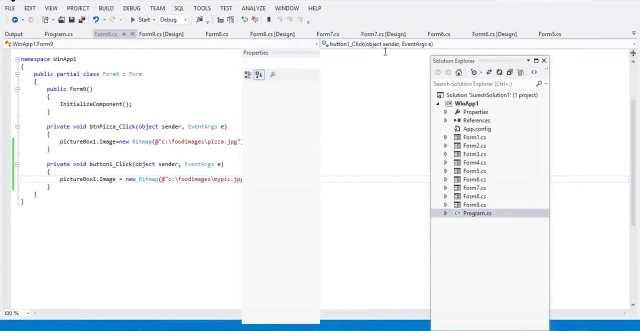 Okay, Let's see this. So I have two images. Let's click on an image. That is, If you want to use double slash, you have to use Add the red symbol. If you use add the red symbol, it will be called a. 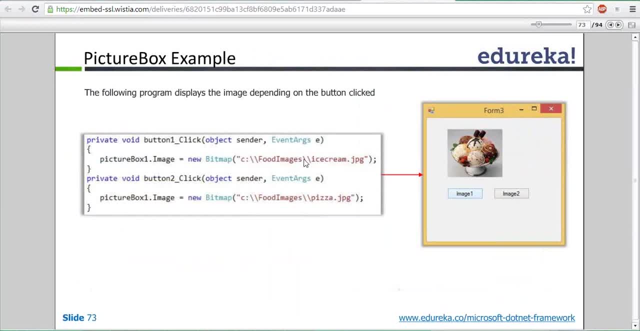 But a back in literal, Okay. It removes the functionality of the slash and uses that as it is Right, One second, Okay, So I have two images Let's click on. I'll. Okay, So I have. 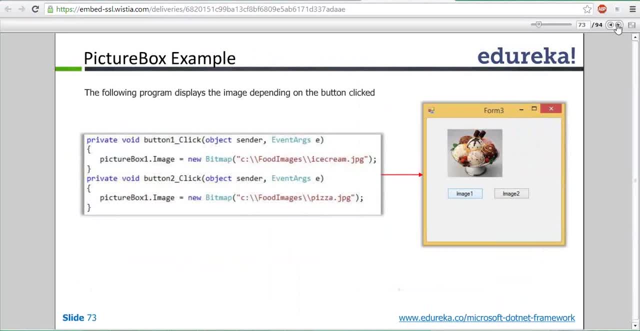 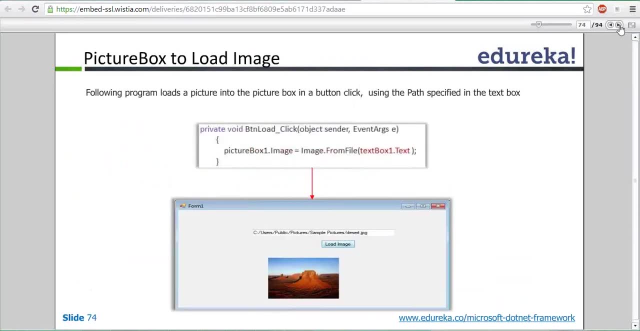 Let's click on Let's Okay, So I have Let's. Let's. Let's Okay, So I have Let's One second. Okay, Come back here. See Image. Do the path.